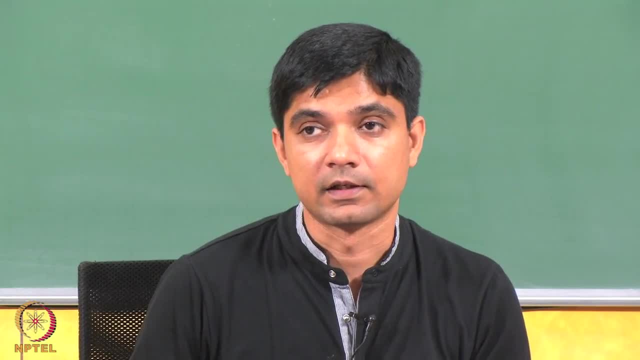 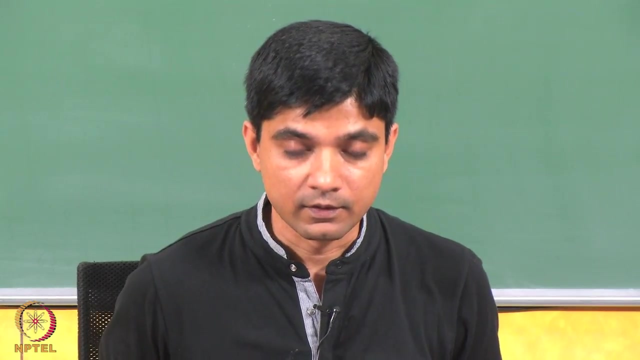 on transfer functions. If we have systems which are interconnected transfer functions, then we had techniques of how to get Create the overall transfer function via block diagram reduction or the signal flow graph techniques. ok, So what we will learn today is once I have a model. So what could? 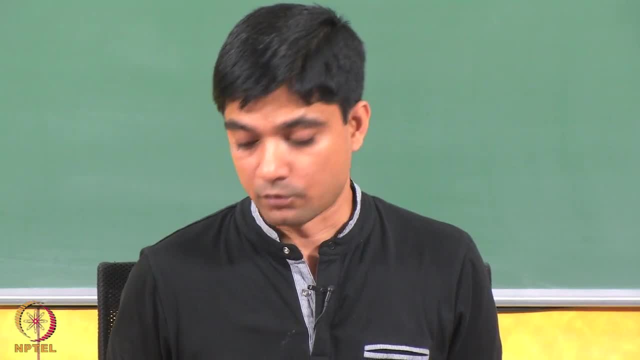 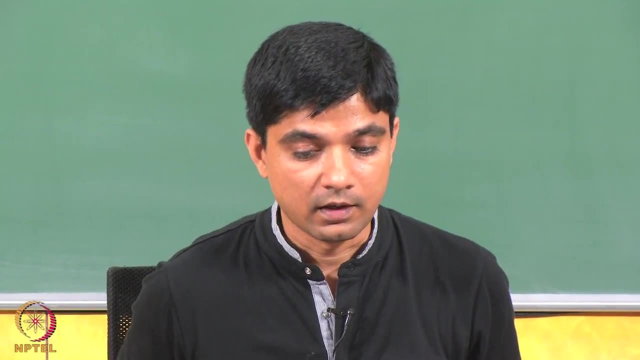 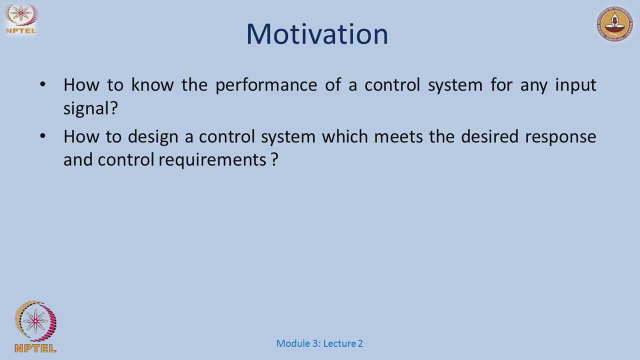 I do with the model, or how does the model behave? So the first thing is, after I obtain the model, how to know the performance of a control system for any input signal, and next is how to design a system which meets some desired response, and it could just be some. 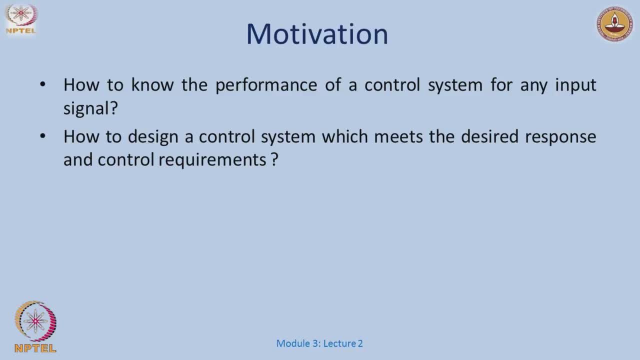 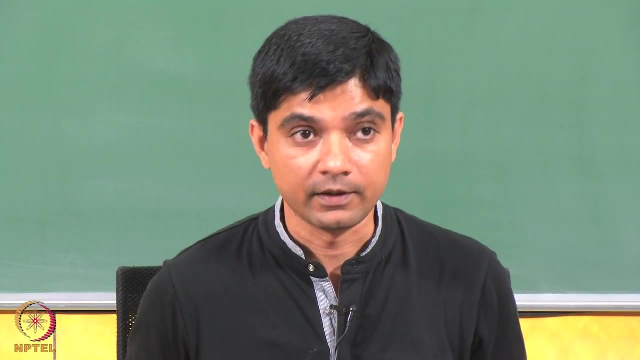 natural response, or even to fit a control requirement. ok, So how do we visualize this? So given a system or given a model? so let me say, when we are subject to driver's license test, right, So the driving inspector does not really. test us for Eheheehagen. 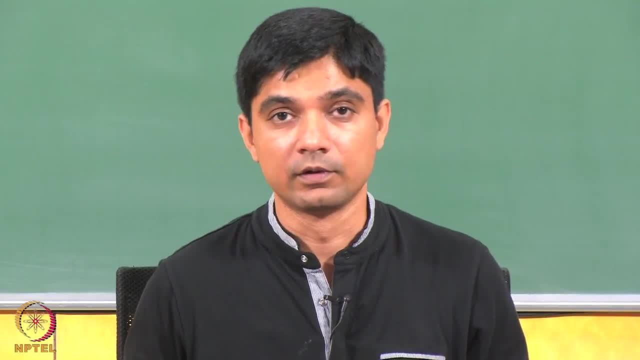 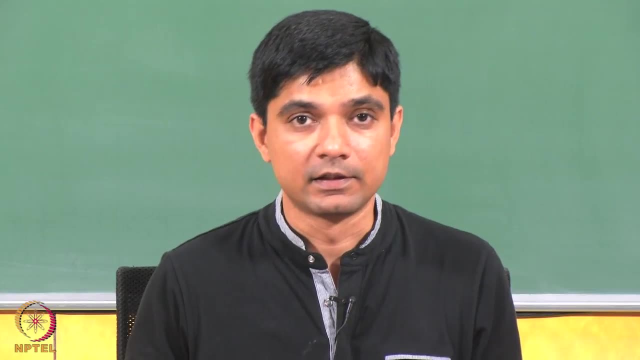 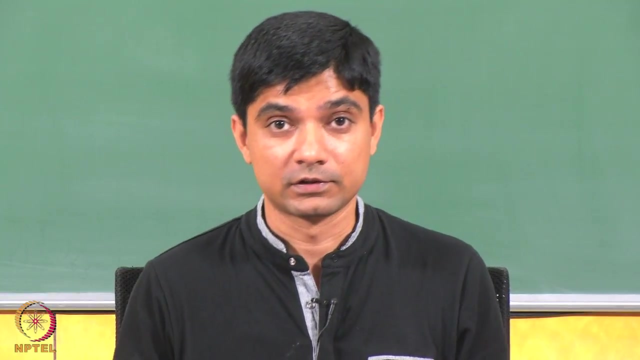 for all possible conditions on the road, which could include high speeds on freeways. it could include heavy traffic on the city lanes. it could involve chaotic traffic with buffaloes running around, kids playing cricket on streets. we do not get tested for all those things. 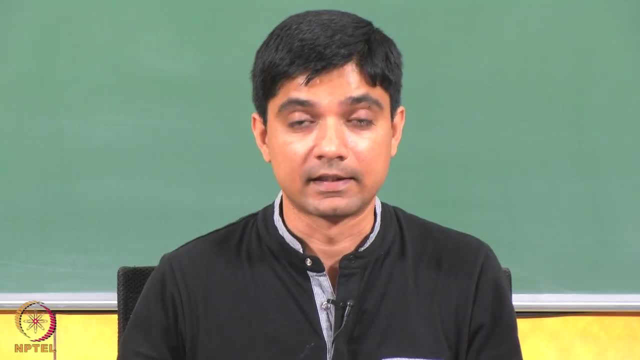 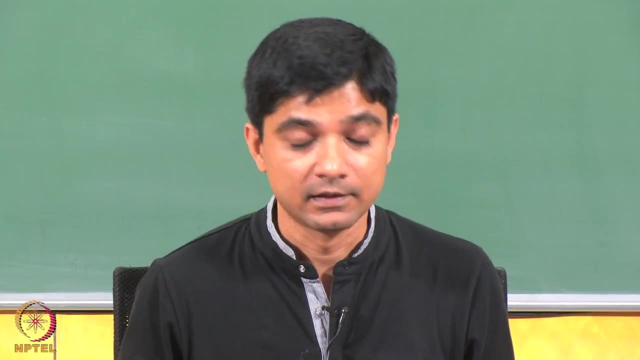 right. So instead, what the driving test does is under standard Indian conditions. So you will just have a little predefined track which you have to drive to pass your learners test. In that track you have several things right: you have to go straight, you have to take, 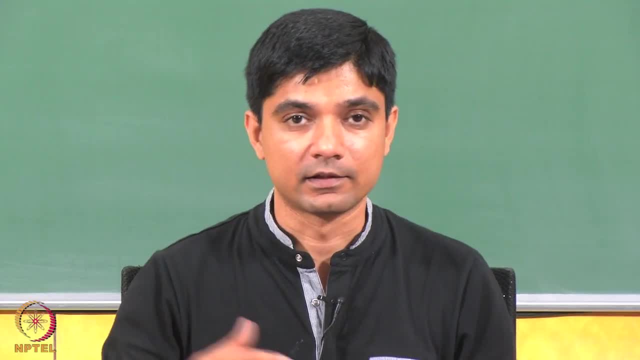 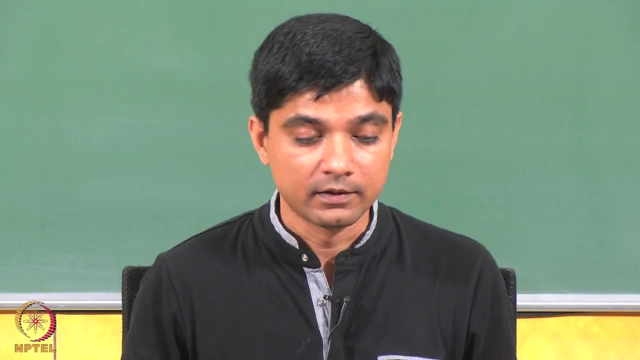 a sharp turn, you have to make a pitch figure of 8, you have to take a reverse, you have to park and several other things. So these are the standard things which we will encounter while we drive on roads right. In the similar way, if I am being interviewed for software, 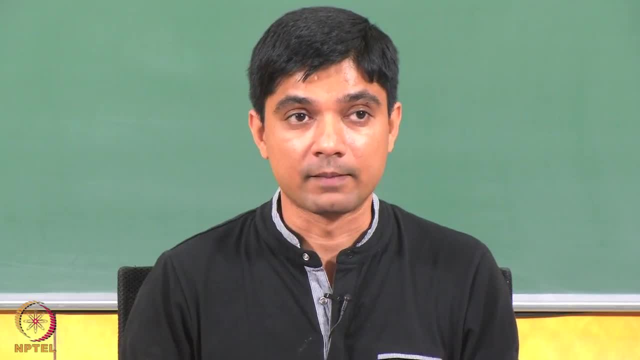 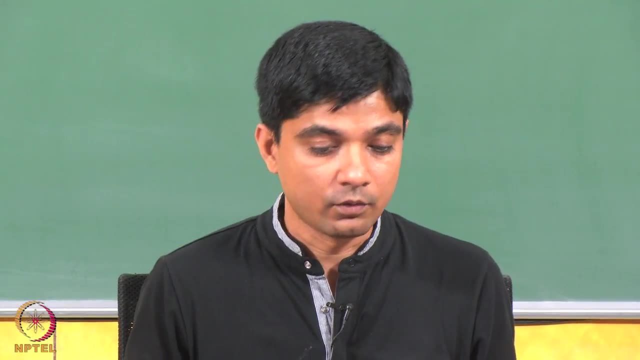 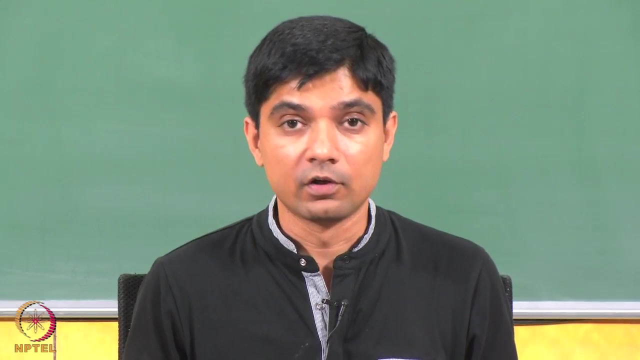 engineer, right, So I go as a model. then my model could be my BTech degree with a CGPA of 8.65, with the several list of courses. Now I want to want to hire you as a C programmer- right, So I will not give you a real time project. 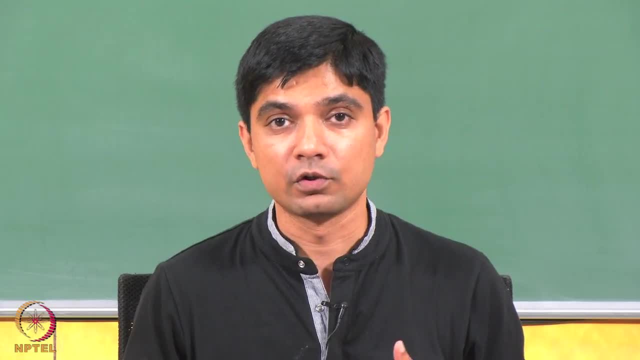 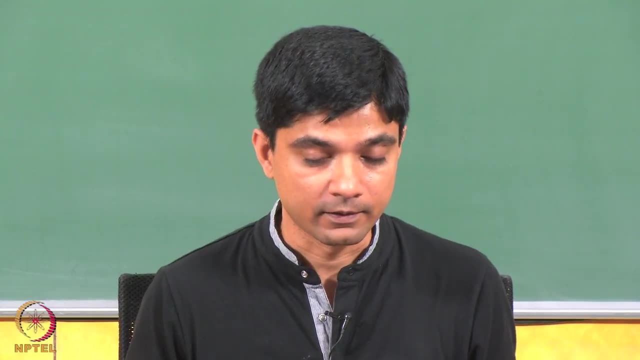 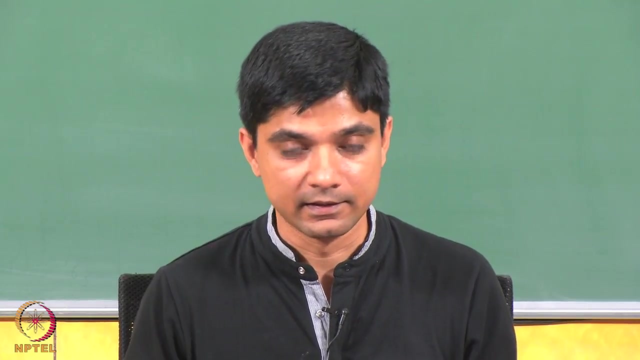 to work on immediately, right? or I would also want to test how would you react or how would your performance be on a certain project or a certain deliverable. Then I would ask you some basic questions on sorting algorithms. it could be things related to pointers linked. lists some functions: interconnection with the data. So these are the basic questions. Ok, So let us now move on to the next slide. So, let us now move on to the next slide. So, let us now move on to the next slide. So, let us. 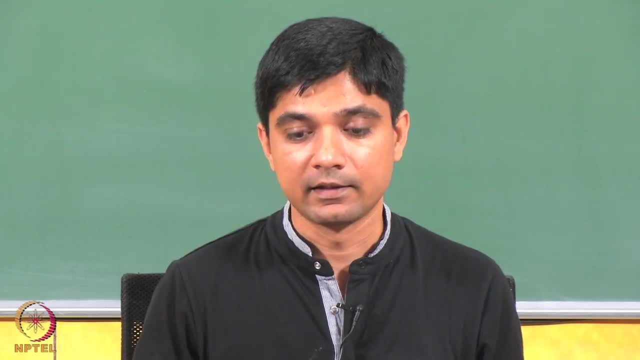 see these things here. So say, daytimeassing the driver, the passenger, the mobility officer, age data, size of your Zoe, time, diabetes, the database, and so on, And based on all these things, I will get a estimate of how your performance could be while handling a real time project. 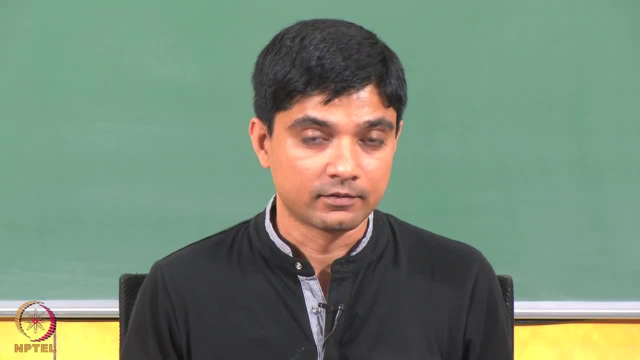 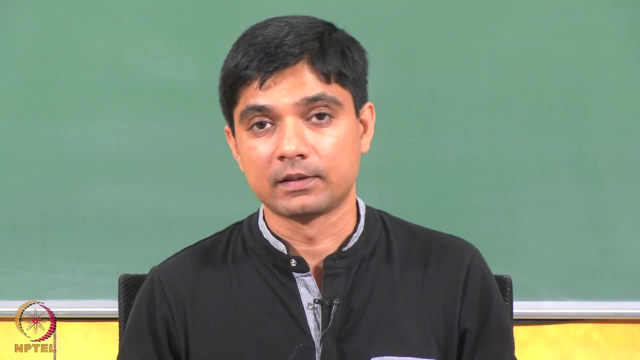 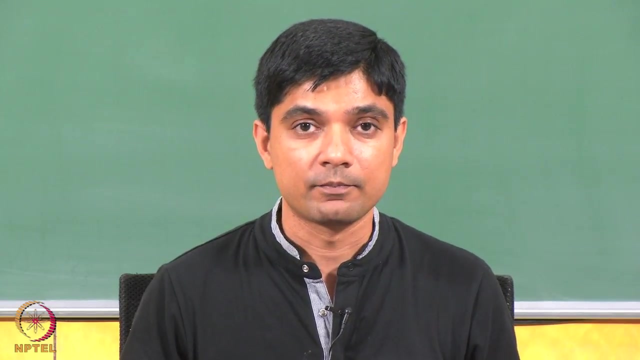 Now this could differ from person to person, right, either you could be a fast programmer, right, you could write a program or code very fast. you could- some other person could take a longer time- but run, write a code which is more efficient. So all these I would get to know with some basic standard test signals. 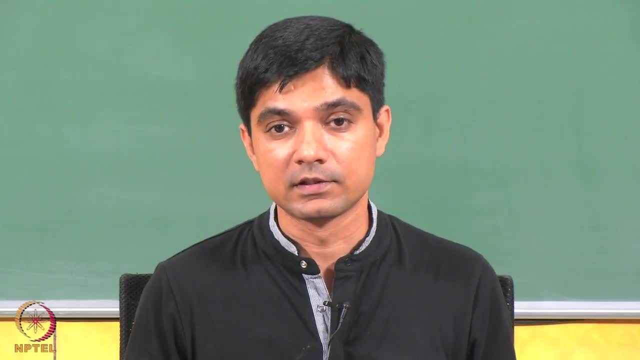 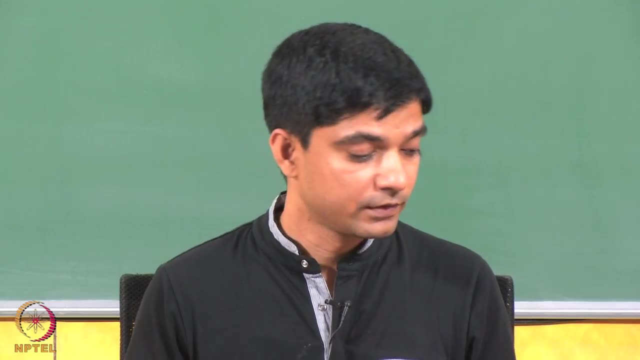 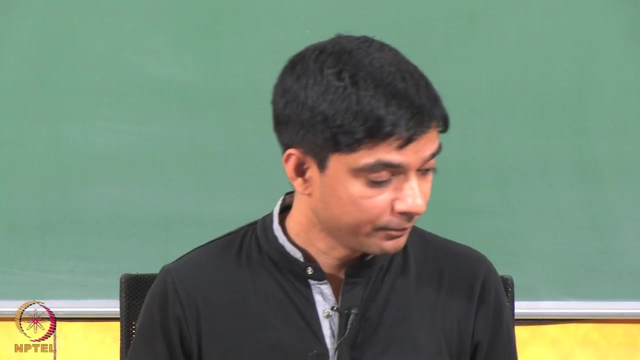 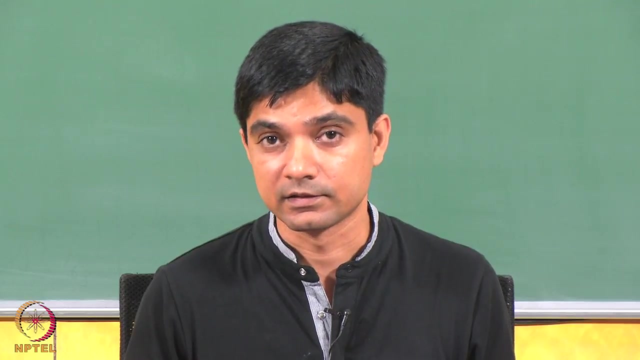 Similarly, what will happen is when we design a control system or we analyze a control system or a model, we will subject it to some standard text signals, because we would not be able to emulate a real time control input kind of signal. ok, So this test signals will tell me how my system will react under changing conditions. 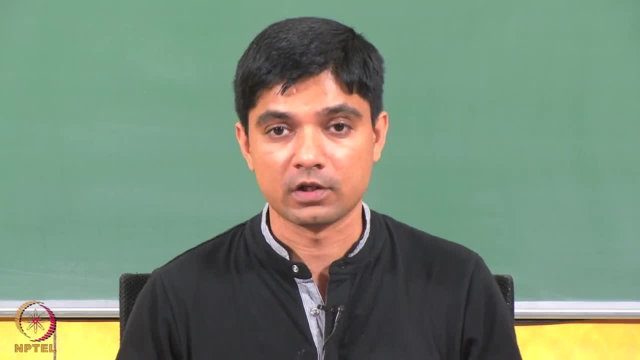 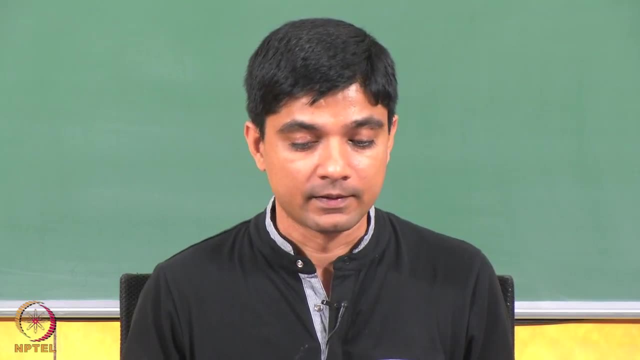 The conditions for a system could be well. I have kind of a shock which could be an impulse test. I could have a time varying signal which could be modeled as a ramp signal. I could have just a sudden disturbance which could be tested with a step signal, and so 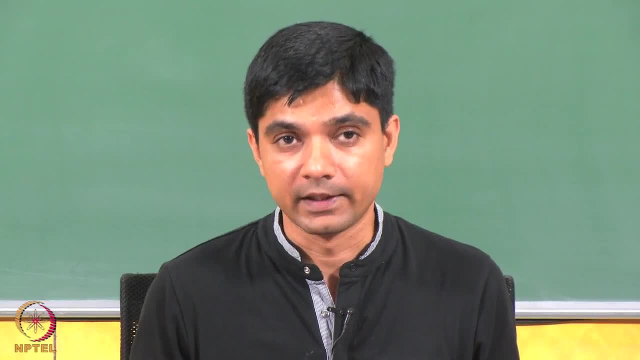 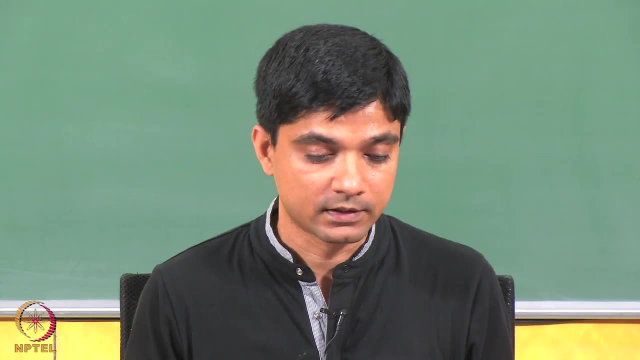 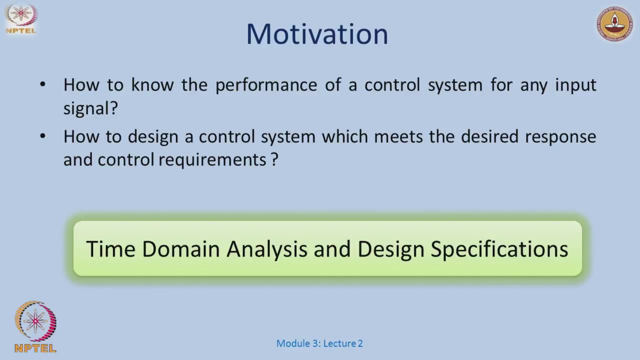 on. So throughout this, we will see how my system would behave. system could be of different nature, right? So how my system would behave based on certain standard test signals. ok, And this will broadly constitute the entire time domain analysis and design specifications. 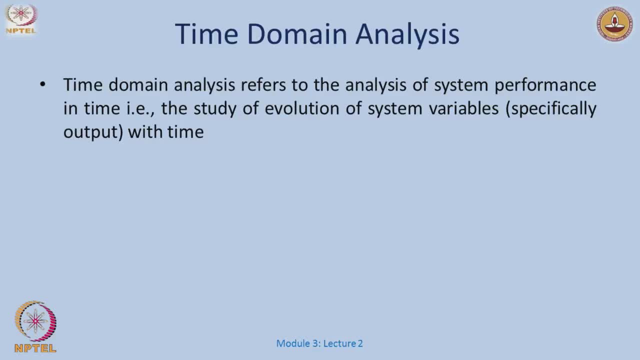 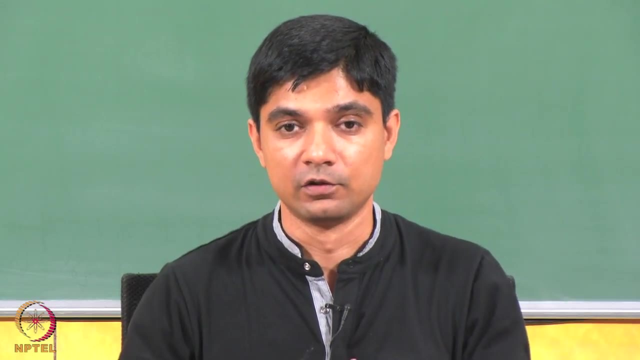 So the time domain analysis refers to analysis of the system performance in time. that is how my system variables, particularly the output, will vary with time, right? So how long does it take for a signal to reach a certain value which I want, like a speed of a car? 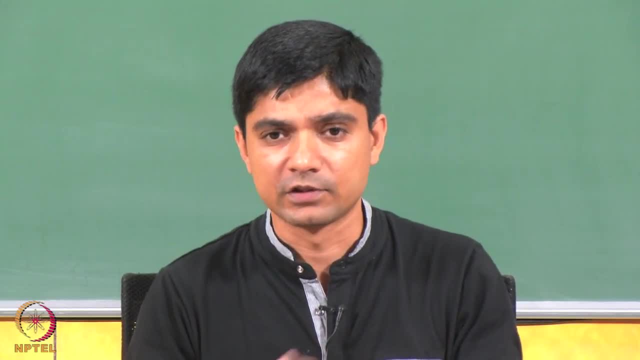 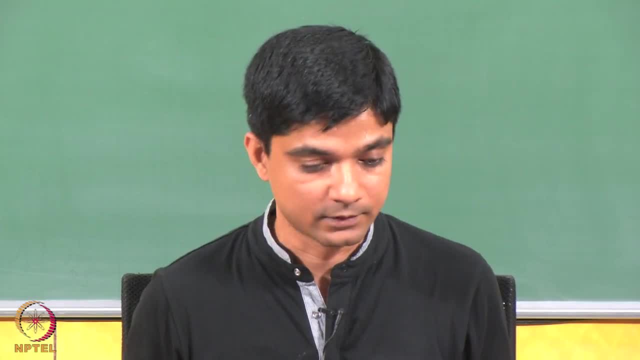 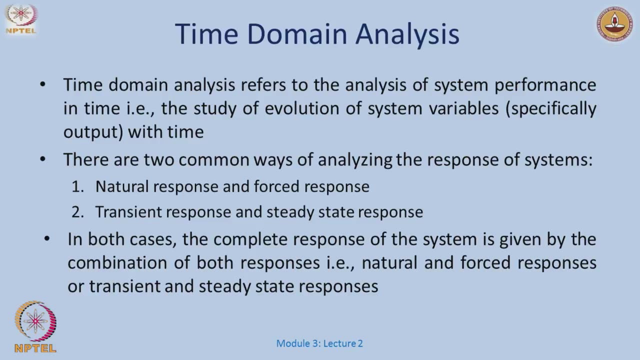 So how? what describes the evolution of the system? variables? ok, So in standard terms, there could be two kinds of response, right? The natural response, and force response, also classified as the transient response, and the steady state response. So I will shortly define what these things mean. 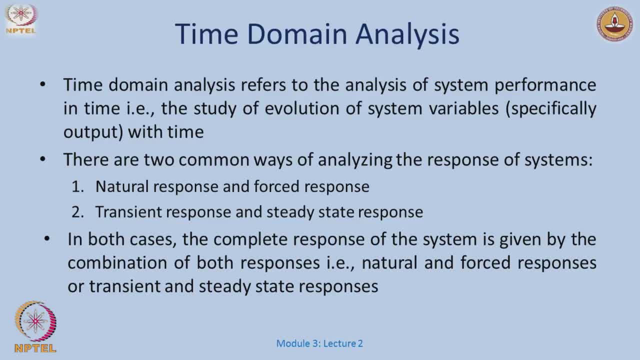 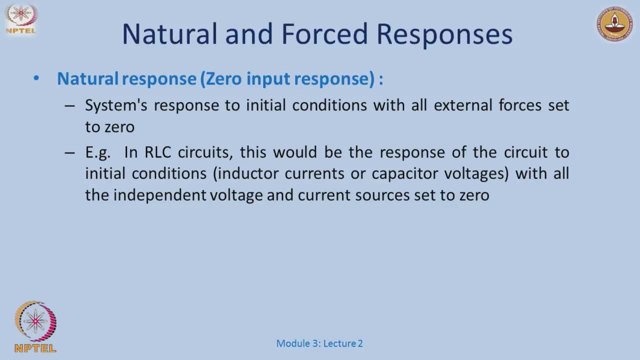 But in both cases the complete response is given by combination of both the natural response and the force response, as well as a transient and the steady state response. right, ok, So what is a natural response It is? it also is referred to as a zero input response, which means the systems response. 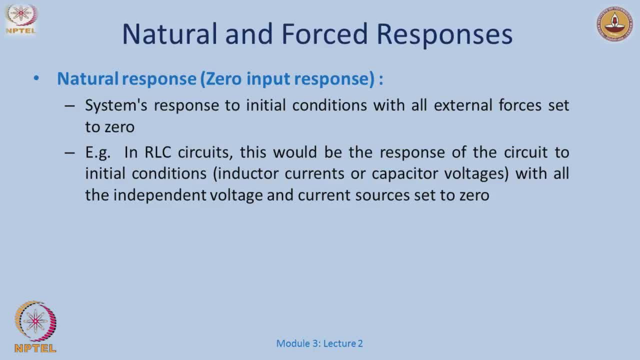 to a certain initial conditions with all external variables. Ok, Ok, So external forces set to 0.. So if I take a simple RLC circuit, this would be the response of the circuit with initial conditions. the inductor could be: could have some initial current or a capacitor could. 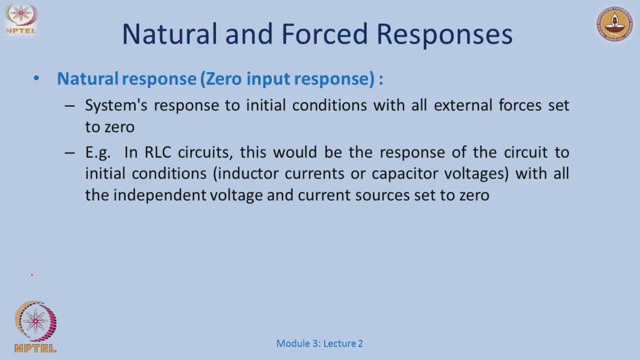 have certain voltage, with all independent voltage and current sources set to 0, which means there will be no external sources. say, for example, I have a capacitor and I have R C with some initial charge, I would call Q 0. The natural response would be that the charge, if I plot with time, or possibly even the current 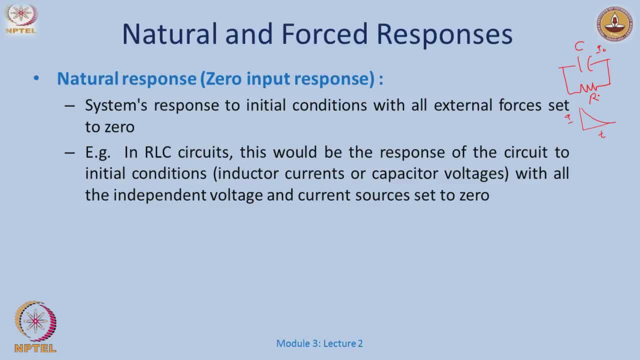 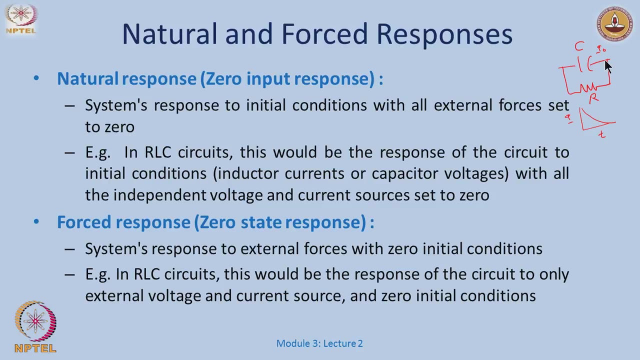 that entire charge gets dissipated through heat energy in this resistance, and that is the natural response. I could then add further elements and inductor with initial charge, and so on. ok, The force response is the systems response to external forces, again assuming that all initial conditions are 0.. 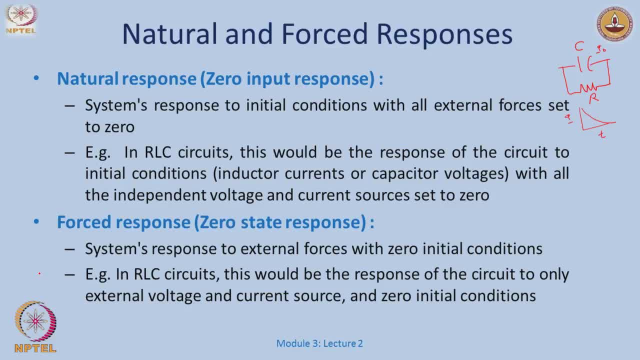 So again, if I look at this circuit, Ok, And I add voltage source here together with the resistance, it will have a different kind of response. ok, We will shortly see what these kind of systems mean and how these kind of responses would look like. right, ok. 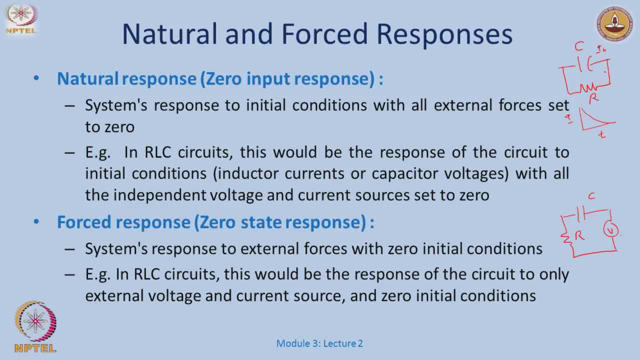 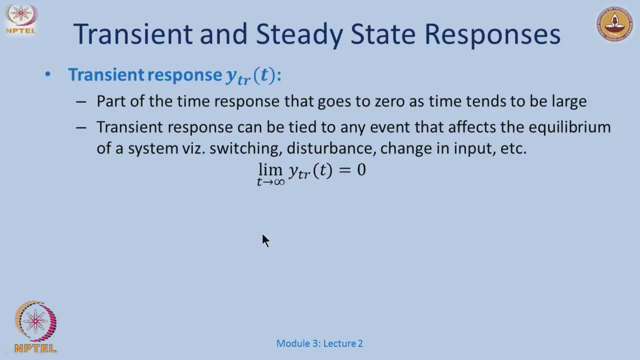 So here there is this external voltage source, here it is. there is no external voltage source, right? So that is a little distinction between the natural response and the force response is also called the 0 state response. ok, Similarly, I have two classifications in terms of the transient response. 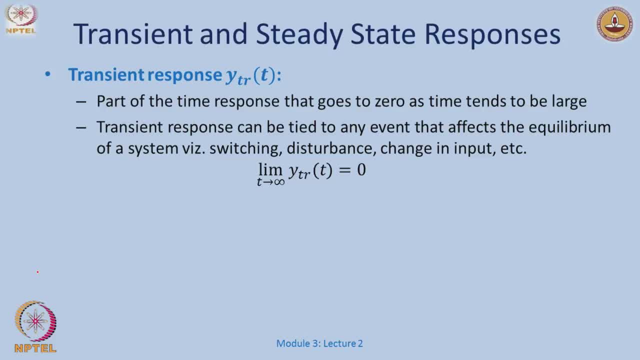 So this, So all this analysis. when I make this for the statements, I would be referring to systems which are stable. right, and I will define formally what is stability a little later. but for the understanding of this particular module, it is sufficient to know the following definition: 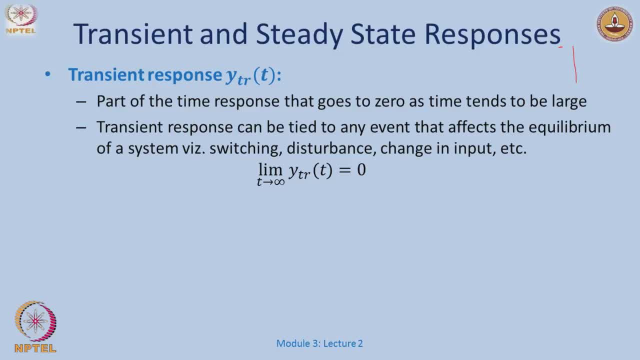 that stability means. So if I am at an equilibrium position, Take my pendulum is just at this equilibrium position. If I perturb it slightly or I start from this initial condition, it will eventually come back to this: its natural state or the equilibrium position. 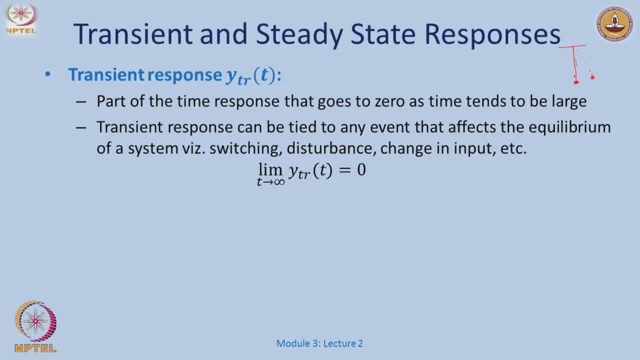 So that, So all systems which are subject to some external perturbation, which then retain their original configuration, would be called as stable systems. that definition is enough for now. right, You can think of it again as simple as the example of a pendulum. 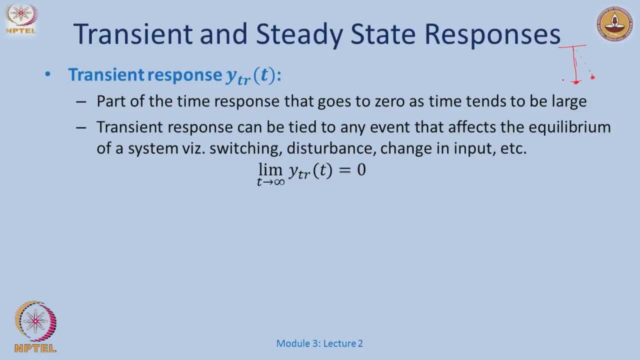 Ok, If just somebody comes and just pushes this, it just goes back to the equilibrium position, same like an alarm clock which wakes you up in the morning, right? So your natural equilibrium position is the sleeping position, and if you have your alarm clock waking you up, that is a little disturbance or a little shock, and then you switch off. 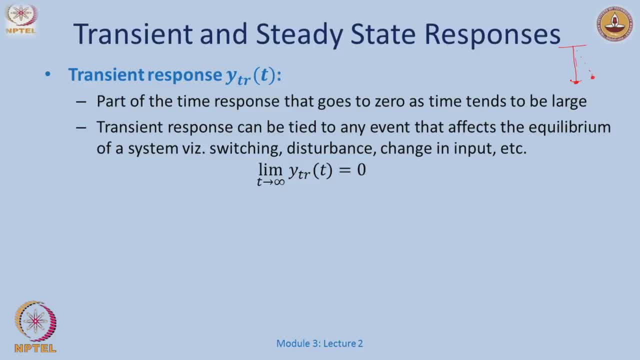 the alarm, put it to snooze and then go back to sleep, which means your stable equilibrium position, which is sleeping position, is always stable, right? ok, So we will talk of. you know those kind of systems. So, in this context, the transient response is the response that goes to 0 or this response. 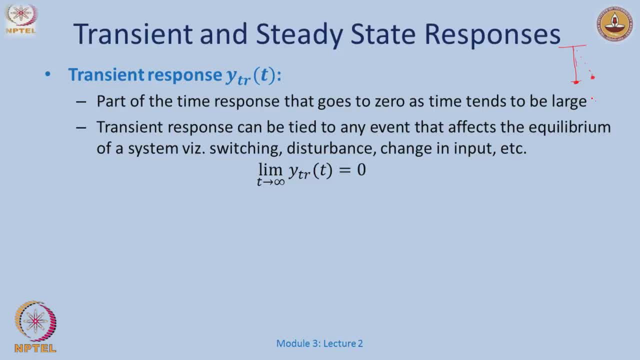 this vanishes as the time tends to be large. So we will shortly see an example with this. It could also be written or it could be tied to any events that affects the equilibrium right. So, as I said in the case of this pendulum right, that the response it just vanishes, as 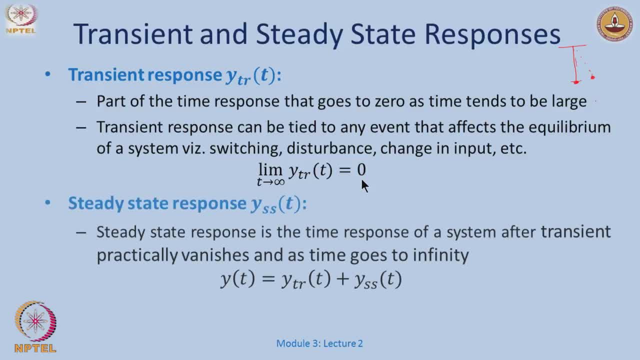 time in goes to a very large value. Steady state response. well, this is the response of the system. after all, the transients have died down right or, as time goes to infinity. again, we will see this with the with help of example. So total response of any system would have two components: the transient response and 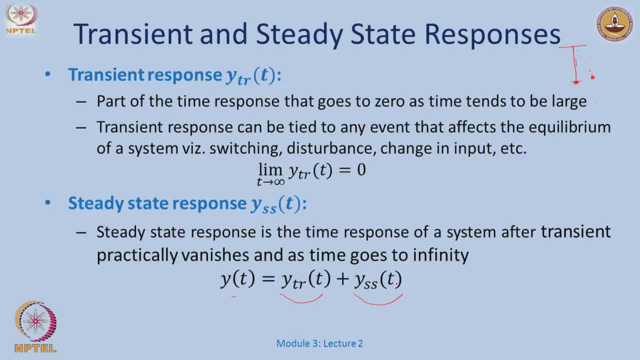 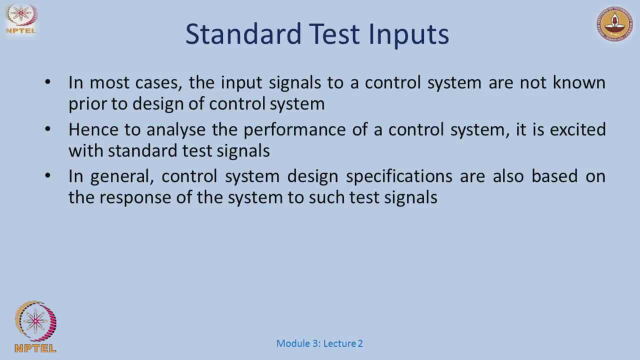 the steady state response, and steady state response could also be just the 0 thing itself, right? ok, Now, as I said earlier that We will, or based on this nature of responses, we will subject our system, or the models which we have, or even the control system, to some standard test signals, right? 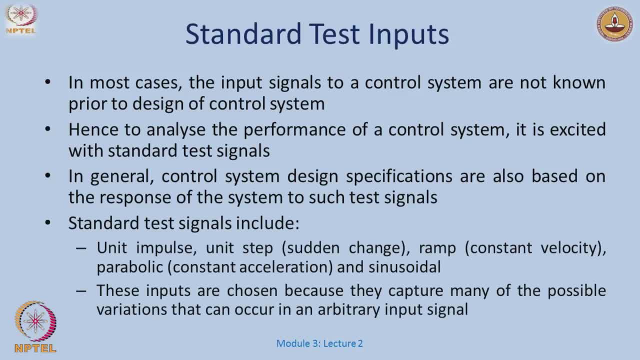 So this standard test signals would be a unit impulse which could be just a shock, a unit step which could be just a sudden change in the system. for example, if I have 10 people in my room with my air conditioner set to 24 degrees, 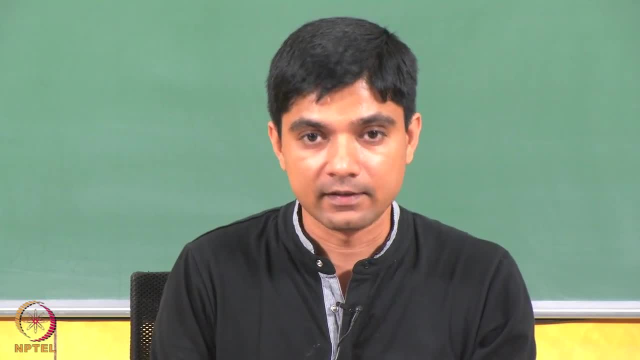 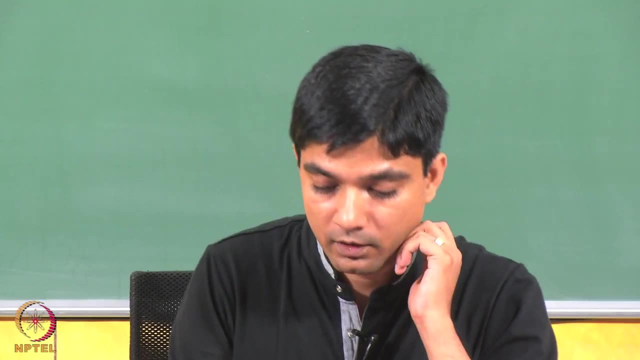 Ok, So these 10 more people add up to the room and just stay there. that is a sudden change, right, it is like a step disturbance. My occupancy is going from 10 people all of a sudden to 20 people, or a ramp or a constant. 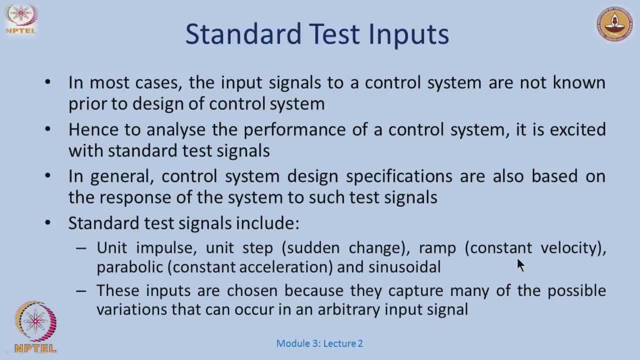 velocity, where you know one person is being added every minute, or parabolic right, which has like kind of a units of, or you can visualize it as something moving with the constant acceleration and of course you can have periodic signals like, for example, sinusoidal signals. 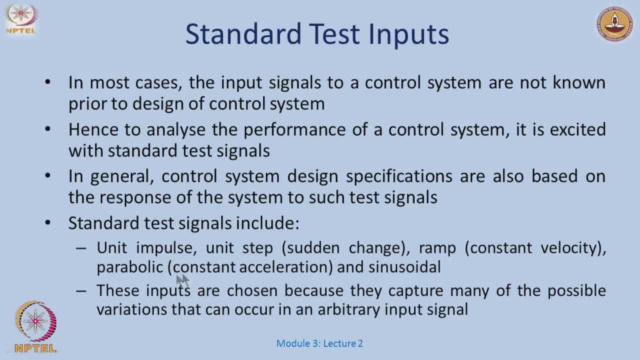 So for the moment we will do analyze impulse, step, ramp, Ok And parabolic signals and postpone the sinusoidal analysis when we will do the frequency domain analysis Again. these inputs are chosen because they capture many of the possible variations that can happen in a real time scenario, right as the driving example or even the C programming. 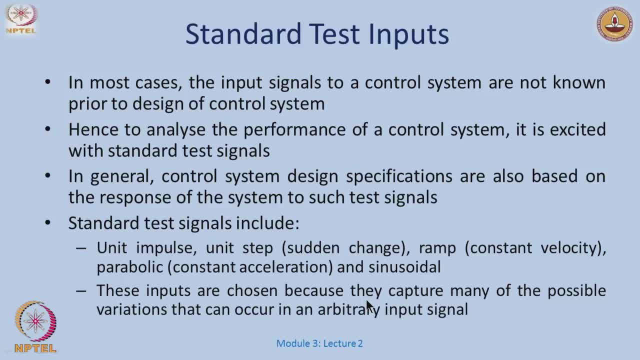 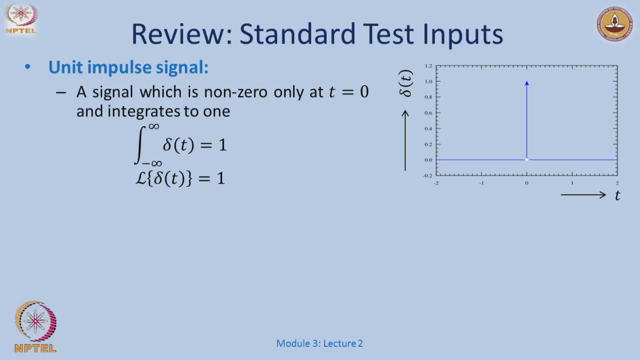 example right And then your. the design specifications could also be based on the response of my signal to a certain inputs. Ok, So just to recall how these signals look like. well, a unit impulse, as we saw and in our earlier lectures, is just signal, for which I integrate from infinity to infinity. the 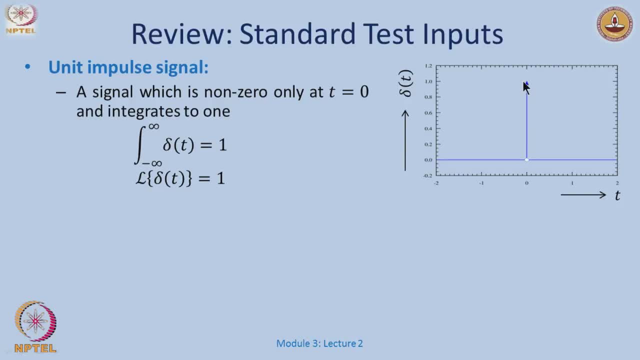 area goes to 1 and it just looks something like this, right? Similarly, step is a signal that switches to 1.. So it just at t equal to 0, plus I am at 1, and then I just stay at 1 and for t all t. 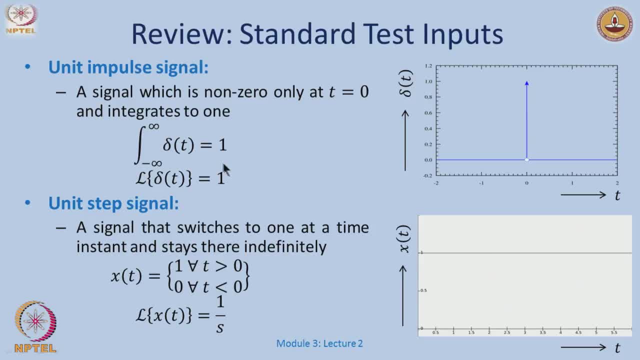 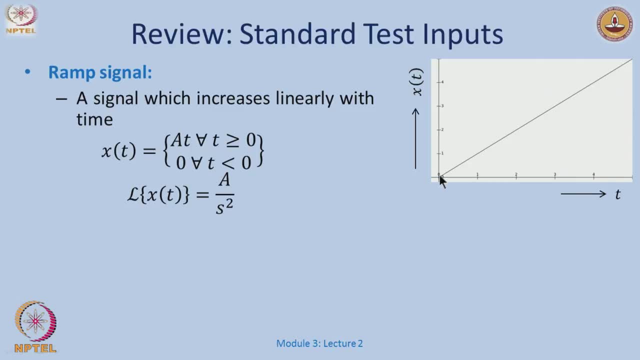 less than 0. I am just at 0, right. So the Laplace transform, we know of a number. Ok, So an impulse is 1 and of a step I know it is 1. over s Ramp is something which is just, you know, with constantly increasing with time at may be. 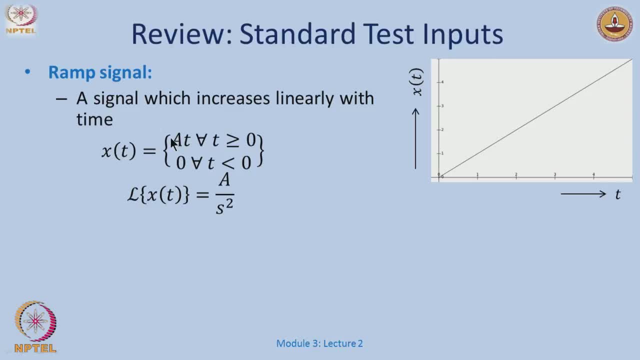 a slope of 1, or it could also be a, have a different slope, depending on what is the value of this a, and then the Laplace transform of this would be a over s square. ok, Similarly with the parabola right. So you have a t square by 2, and then the response increases actually faster than what. 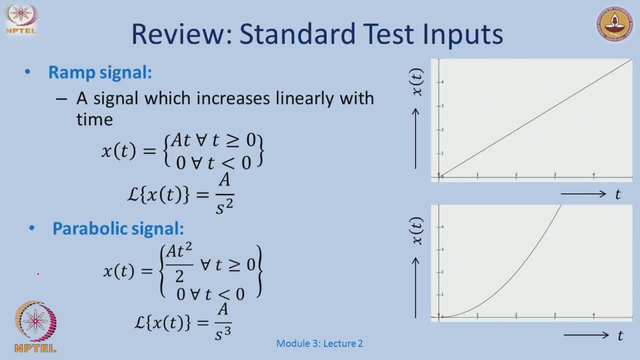 it was here, Ok. So one thing which you could notice is I take this parabola, a t square by 2, and I differentiate it. what I get is a t, ok. Similarly, I differentiate. So this is a parabola, I differentiate it to get a ramp right, that is, you can see it. 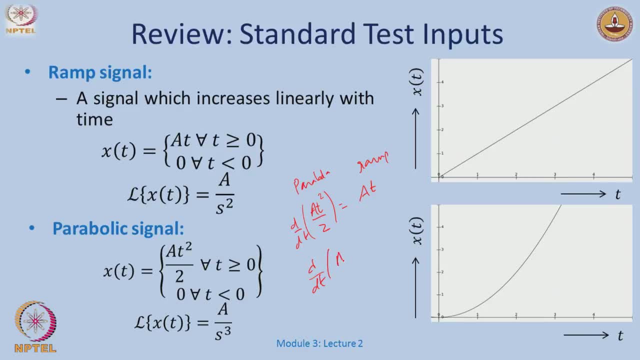 here. Now I differentiate, Ok, So I get a ramp and I get a step right. ok, now just keep this in mind for a while: that I differentiate a parabolic signal to get a ramp, I differentiate a ramp and I just end up with a step. this is a step of size A. Now we will see. does the response also have certain? 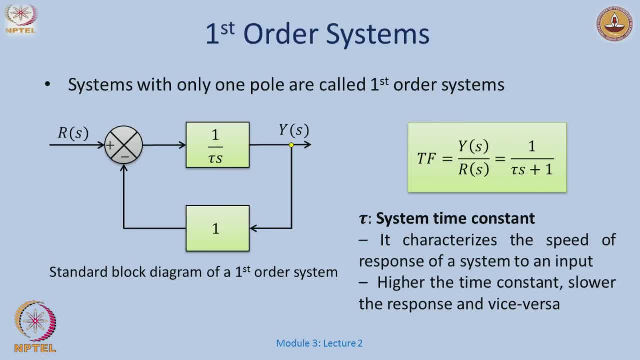 behavior like this. right, We will just see if that is true or not. ok, So the simplest of all systems are systems with only one pole and or called first system. There could be some simpler systems where I just go from here to here. they are just. 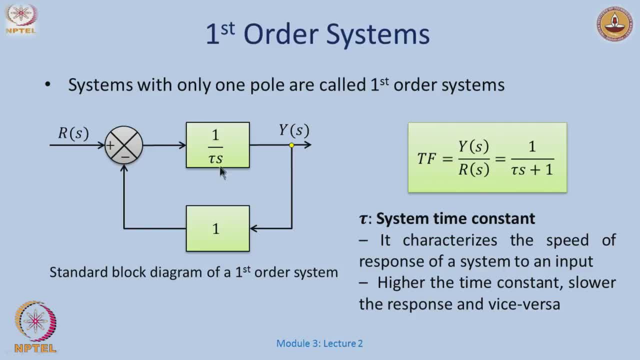 a number 1 and I am not worried about anything, right, So that those are not of interest. there is some dynamics here, right in terms of tau times s. So if I just do the standard feedback interconnection, I compute the transfer function, I just get. 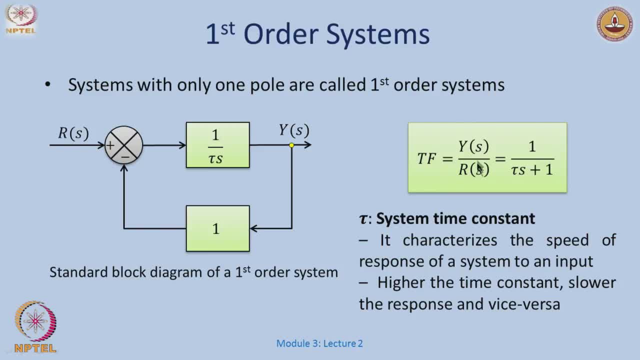 that the transfer function from r to y is y over r is. So I get the transfer function from r to y is y over r is. So I get the transfer function from r to y is y over r is. So I get the transfer function from r to y over r is. 1 over tau s plus 1 and usually. 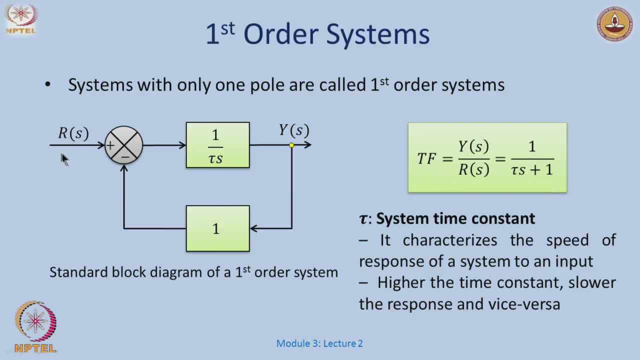 r is could be the reference signal which my system is subject to, and I will see how my system behaves for different reference signals. right, The tau is a system constant and it characterizes the speed of the response of a system to an input, and we will see this with the help of an example. 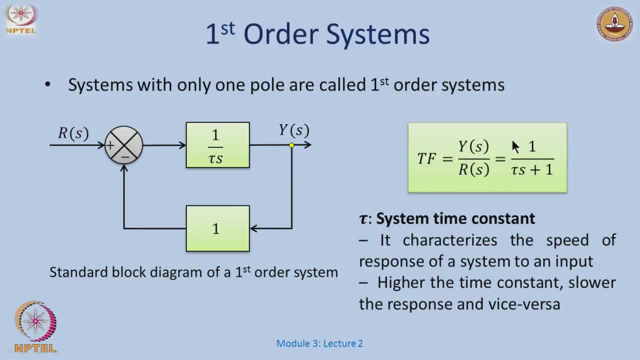 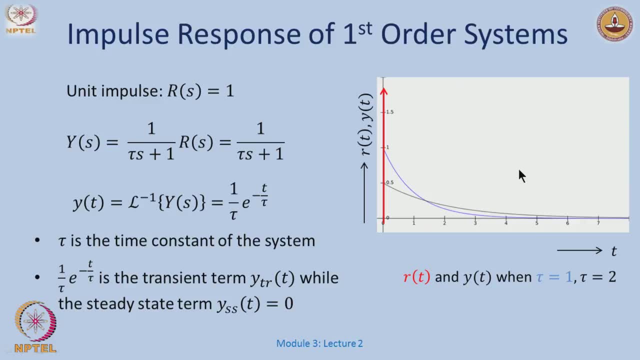 So let us just start with dealing with first order transfer functions, which look like this: 1 over tau s plus 1. ok, So if I just take the input Now, we will use all the tricks which we learnt in, you know, Laplace transform, solving of differential. 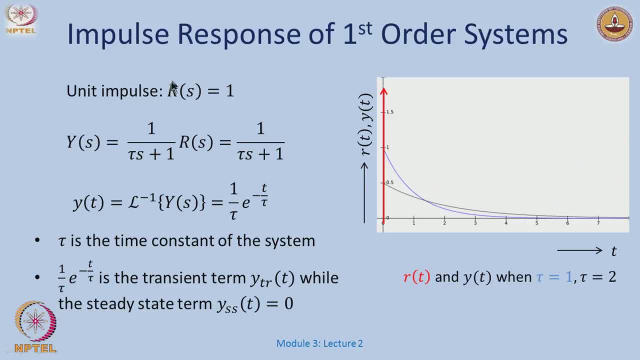 equations and so on. So my input or the reference is just 1 y of s, which is the transfer function. g times r looks like this y of t. I just take the inverse Laplace of this guy and I get this guy right. So 1 over tau e, power minus t over tau, where tau is the time constant of the system. ok, 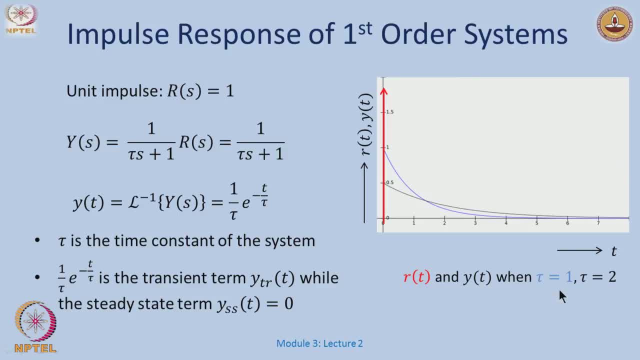 So if I just look at the plots quickly, right? So if I choose a particular value, tau equal to 1, then you know my response just dies this way for tau equal to 2, I have something like this: ok, So you can see that with changing time constants, your response also changes, for example the: 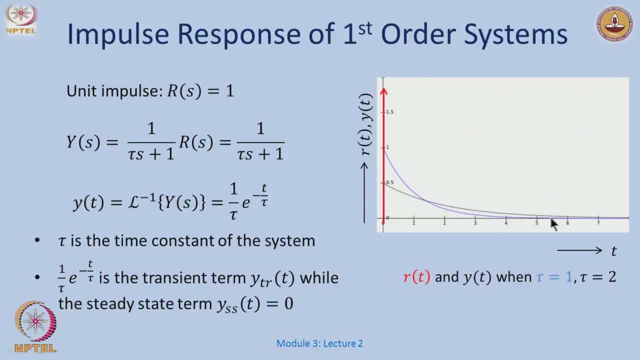 blue line, which has a smaller time constants, approaches the horizontal line faster than the black line, which has a higher time constant. ok, How does it look in terms of the steady state? Ok, So this is the steady state or and the transient response. 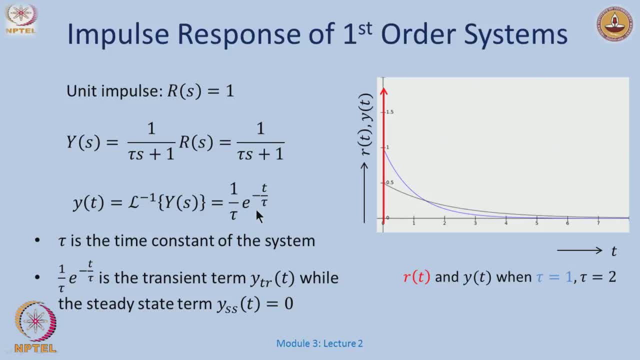 So this guy- 1 over tau, e power minus t over tau- is called the transient term. if you see that, you know as. So how did we define the transient term? that these guys tend to vanish as time becomes very large, right? So as time t goes to infinity, this guy goes to 0 and, of course, the steady state term. 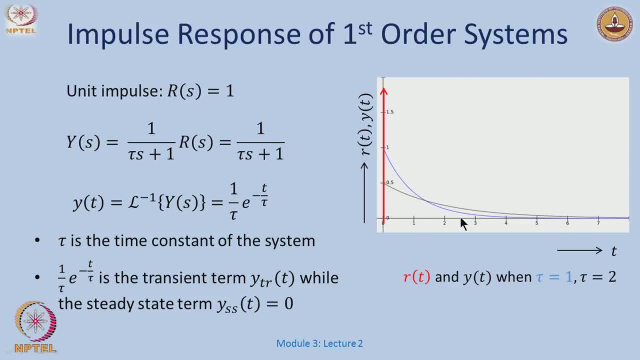 here is just 0 right. as I said earlier, the steady state could term that the y eventually. So what the term or the value where which the transient term steady state, Which the transient term settles down, could actually be the steady state value which is? 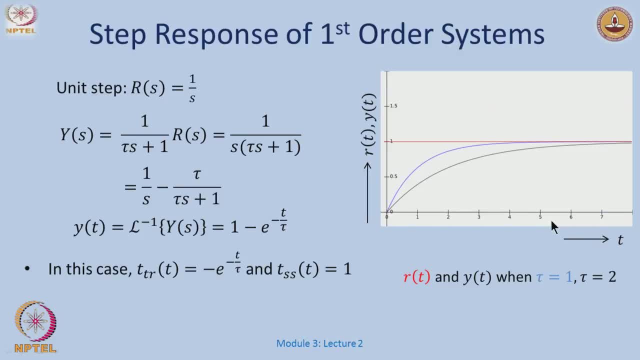 true in this case. ok, Now I go slightly further. right, I look at the step response, or when you see more simply a unit step, I can change the magnitude, but nothing much changes in the analysis. So y of s is again. the transfer function is just a first order transfer function. the 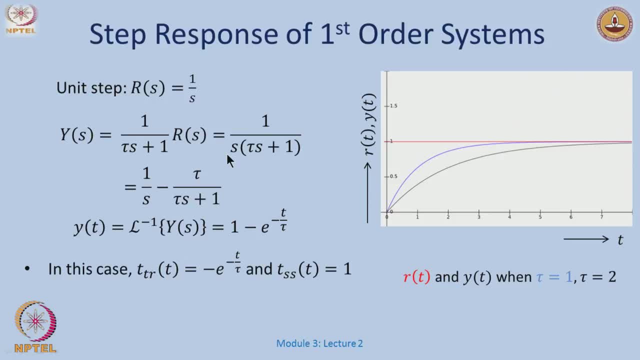 reference is a step, So my overall output would look like this: ok, Then I do some tricks, Ok, Ok, So let us do this here and get the inverse Laplace transform as 1 minus e, power minus t over tau. it is something different here than what we had learned earlier. 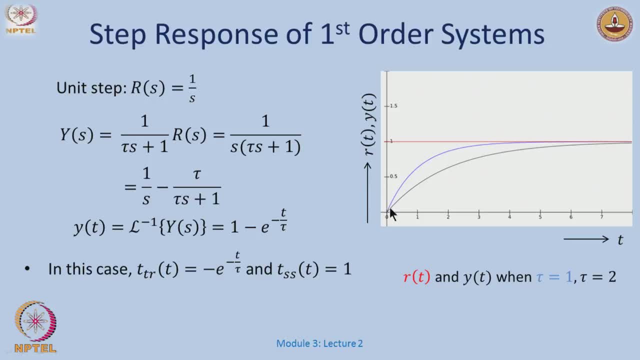 If I just plot this for two values, say, at tau equal to 1, I start at 0 and I go and I end up at 1, asymptotically or eventually. I take tau equal to 2, I still end up at y equal to 1, but a little slower than before, right? 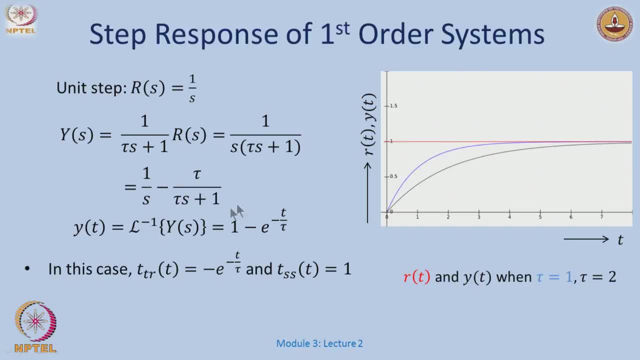 So in this case there are like two terms, right, So this is a term which vanishes as at infinity. right that the transient term, and this is the steady state term, right At steady state. what remains is only this: guy 1 and at steady state, if I just write. 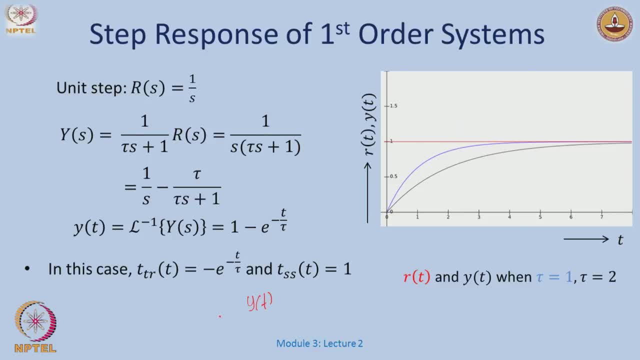 that down y of t limit t going to infinity is 1. ok, So let us see. So, let us see, Ok, So I could also compute it directly from here, right, just to see how the steady state looks like. I can just use the final value theorem right, which goes limit s tending to 0, s times y. 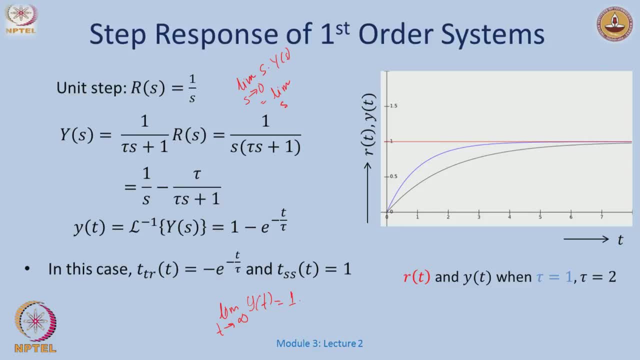 of s is limit s going to 0, s times 1 over s tau s plus 1, these guys vanish and I am just left with 1.. It also is in agreement with what I get here and system is stable, So I can always use this. 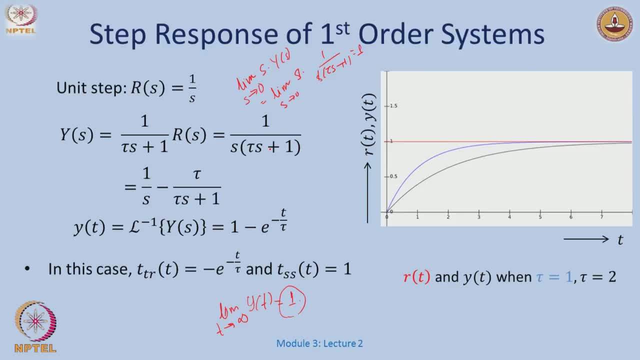 Ok, So this is the final value theorem, right? So I have here. I have a transient term I can see very explicitly, and the steady state term, which is actually non-zero. In the previous case, the entire response was just going to 0. ok. 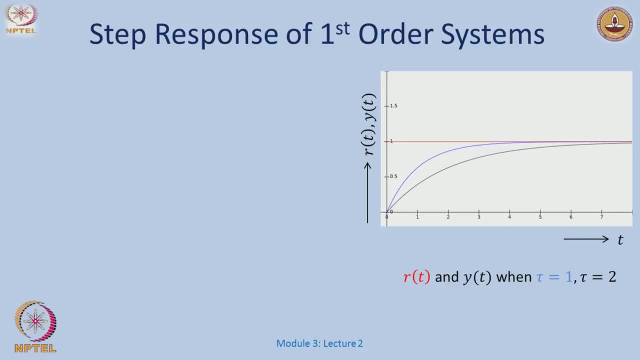 Now something good happens here, right? So look at this signal. right? So what I have is y of t is 1 minus e power minus 0. Right, So what I have? Ok, So y of t is 1 minus e power minus t over tau and say t equal to 0, y of 0 is 0 and 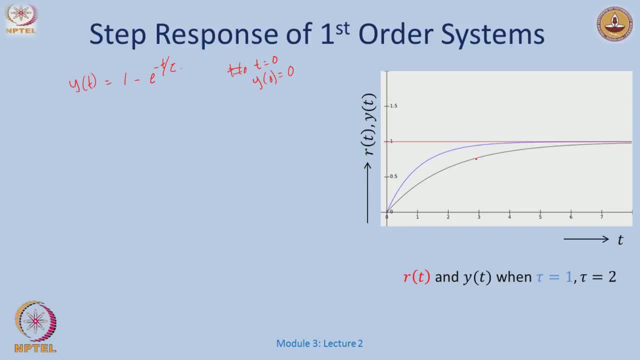 that is what the even the plot says, and at t equal to the value of the time constant I have y of t is 1 minus e power minus tau over tau. So I am just looking at: 1 over e power minus 1 is like 0.63.. 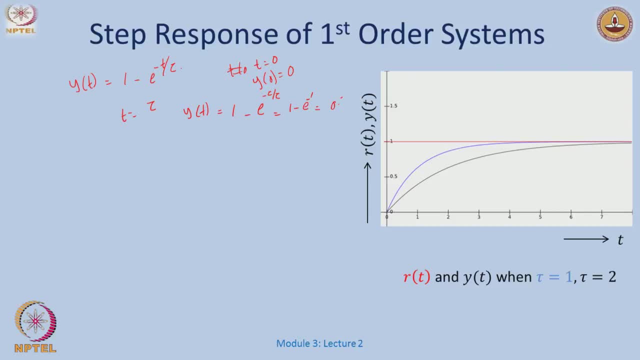 Right? Ok, So y of t is like 0.632 or 63.2 percent of the final value, right? So what I could observe here is: let us say what happens. even as t equal to 2 times tau, I reach. 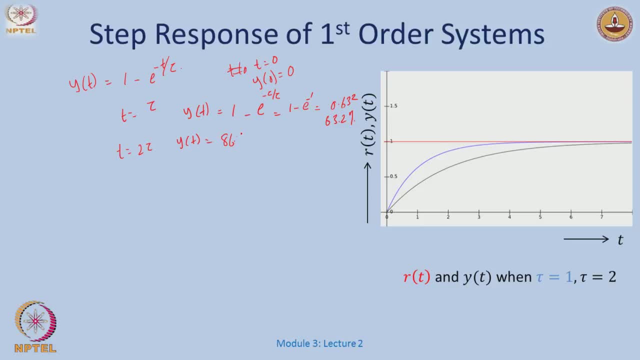 So my y of t would be 86.5 percent of the final value. I do it for 3 tau, So y of t is 0.632.. Right, So y of t at this for this t would be about 95 percent and at 4 times the time constant. 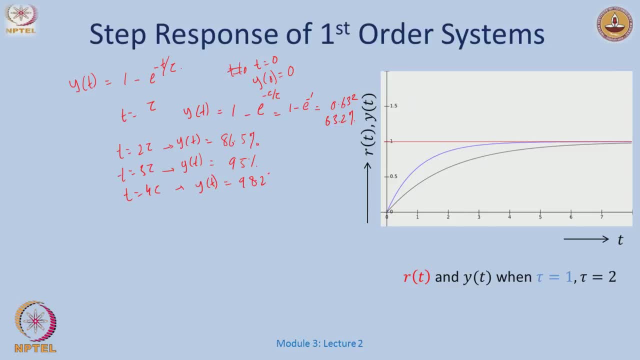 I have y of. t is like 98.2 percent of the steady state value, which is 1.. Right, Ok, So I can just plot this here, that at t equal to 1. I can just so for the for the blue line. 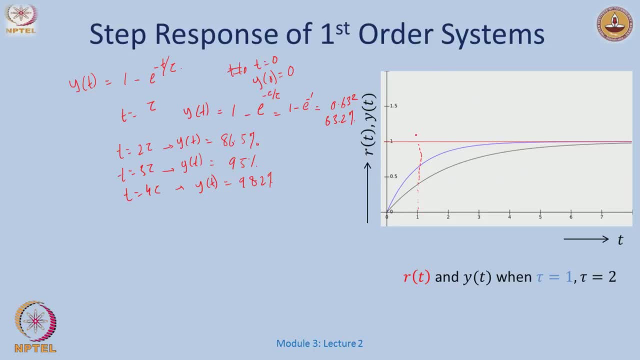 this will work nicely here, So I will just be somewhere. So this is, this is like the 0.632.. Ok, So few things to observe here, right? So one is: let us see what decides this, if who goes fast and who goes slow. 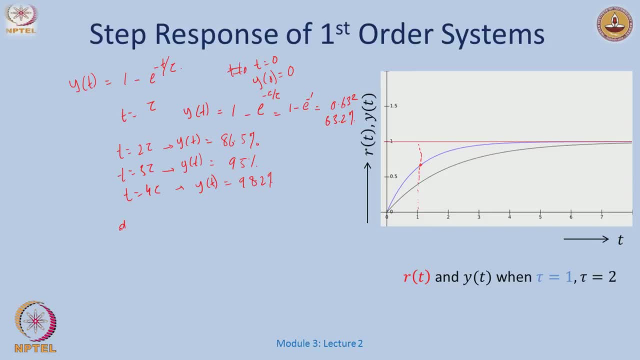 So let us try to differentiate this signal. right, So I have d over dt of y of t, that is. So I have 1 over tau e power minus 1.. Right, Ok, So tau e power minus t by tau. 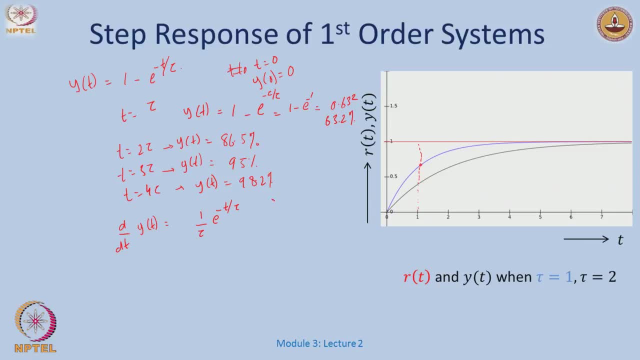 Ok, Now at t equal to 0, so d over dt of y, of t is 1 over t. Ok, So the initial velocity or the initial speed here is of a slope, 1 over t, and then just goes on, and this just meets this point here. 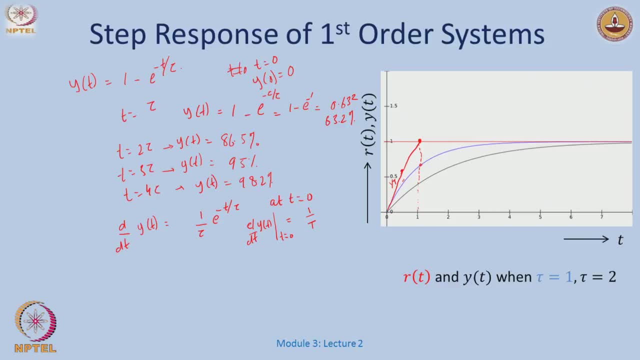 Right. So if I keep on going at the speed of 1 over t, I will hit this point exactly at t equal to tau, Right At this. this point, which is my time constant I have. similarly, if I go So here with the speed, it will be at t equal to 2 that I am putting this value. 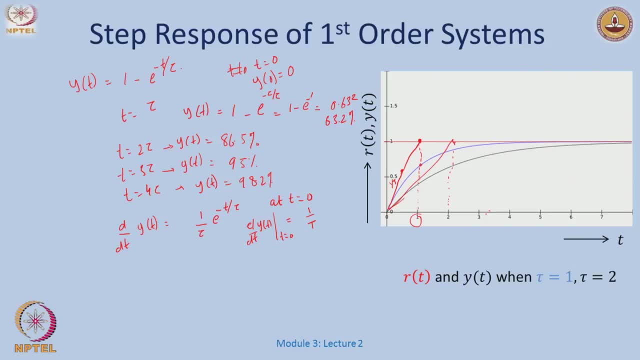 Right, Like this, This and then this one. You can compute it right for different time, constant- this is a general formula for that- And of course, the slope keeps on decreasing, Decreasing, Decreasing And so on. Right, So ok. 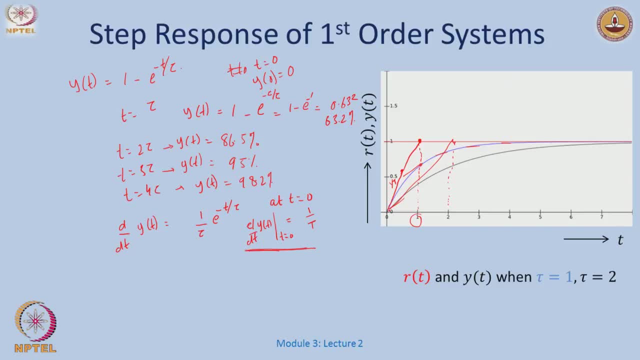 Why is this important? and then why cannot I, you know, maintain this speed all the time and just go to 1 in 0.6 seconds than just you know going this way? Well, this phenomena, essentially, is because of the dynamics of the system which gives 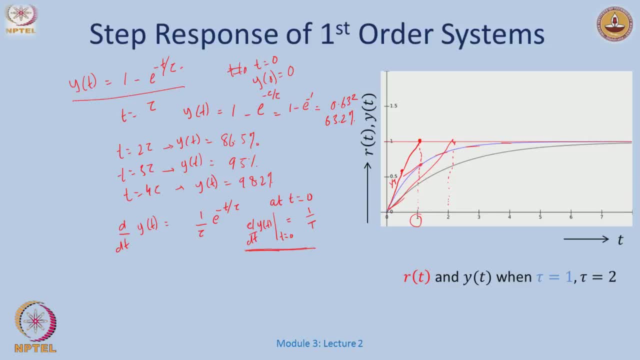 you a response like this Right Now, this curves could be explained by what is in here. So this we could. this is something what we also experience in our daily lives. Right, If I take an, an an elevator from from, say, floor number 1 to floor number 6.. 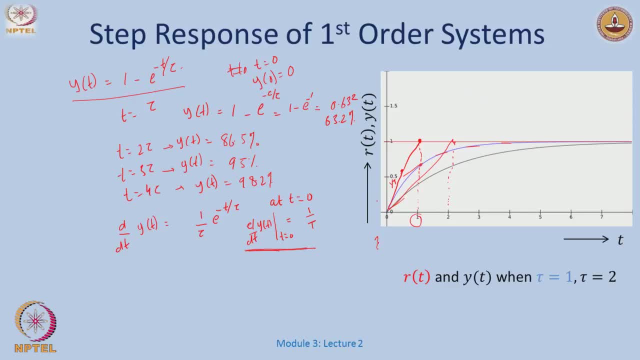 You see that the initial velocity is a little higher, and then, as it goes up and up, you do not have the same velocity all the time, until you reach the 6th floor and then abruptly come to a stop. You go, you keep on going up, up, up, up, and then the velocities keeps on going down and 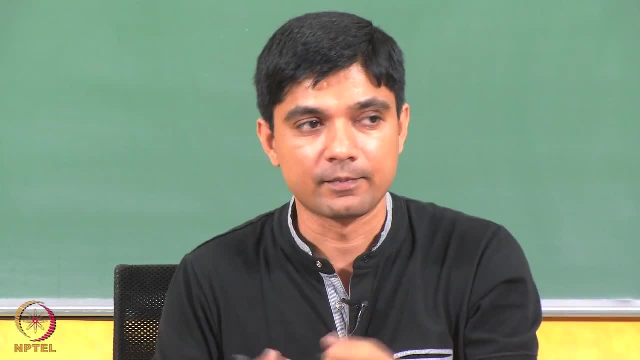 then you just stop at the 6th floor very gradually. the same even when I am driving a car from point A to point B. Right, I build up a velocity and then I just I just do not go and hit that point and then stop. 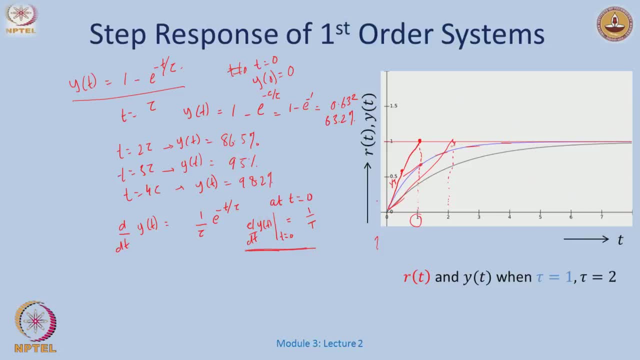 abruptly, Right? So this is a phenomena that could be explained, you know, in that kind of fashion, Right? And then this: if you look at this slope also decreases monotonically as t goes to infinity and until it reaches slope of 0. 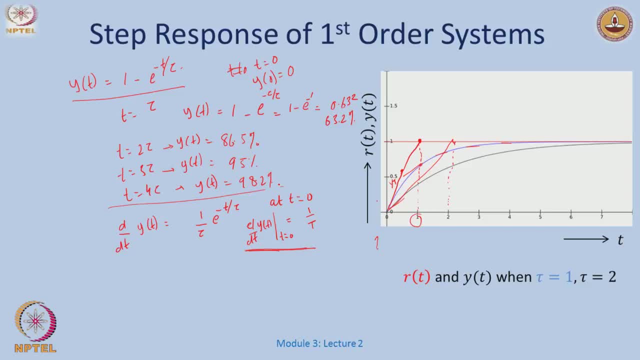 Now, what about these guys here? How do? how would I say that I have actually reached some kind of a steady state value, right, I do not have to wait till infinity. So how do we define? is, if I say of what I will slowly define, a term now called the settling. 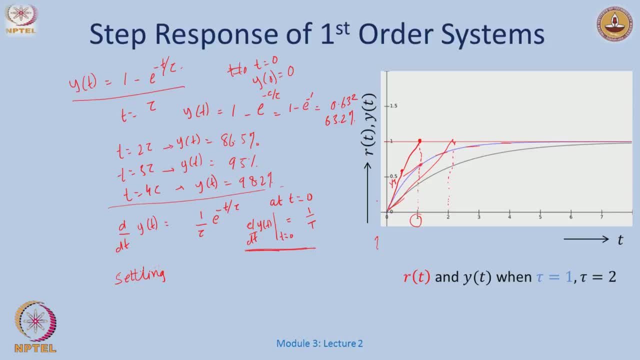 time Right, Or when I would say that my system has actually reached the steady state, is when I am within 2 percent of the final value Right. So if I reach 0.98. Like, for example, after 4 time constants, then I say that my system has actually reached. 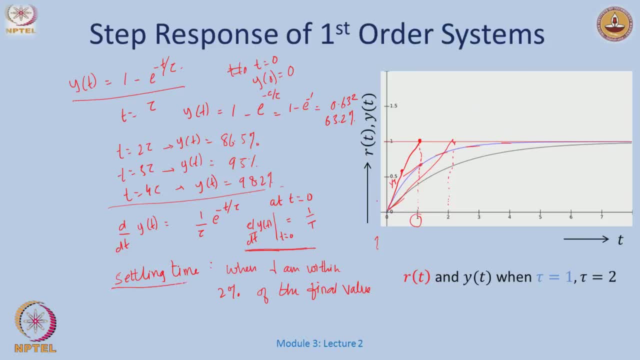 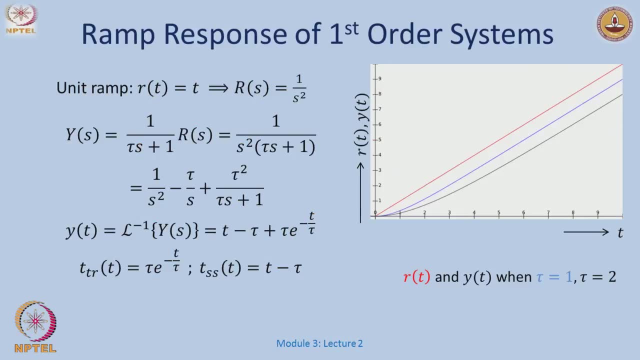 a steady state. This is. this will be very useful for analysis purpose, right? this definition of settling time, Right, So ok. So after this, well, you can look at the unit ramp response, Ok. So, even before I do this, 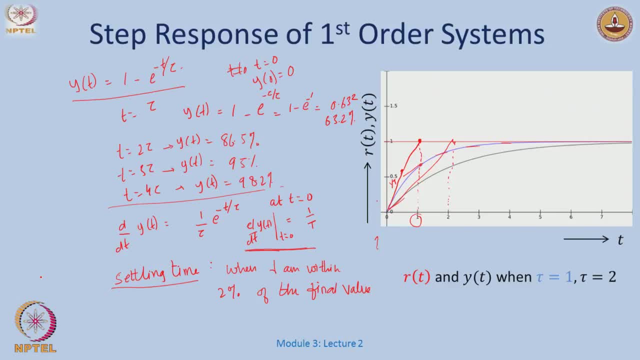 Right. So let us let me do something else also here, right? So here my reference was a unit step, if I just look at the standard configuration. So I had. I think, if I just remember correctly, it will be 1 over tau s. I had unit step. 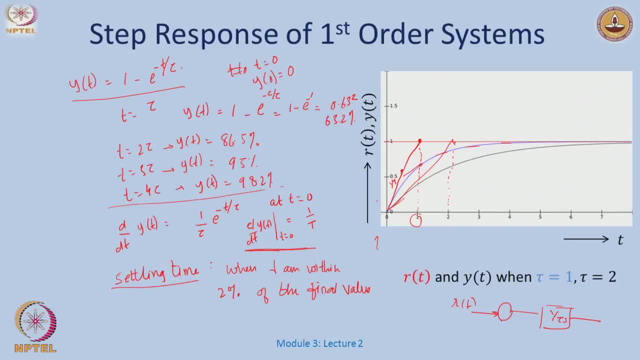 here, which was my r of t, this right. So y of t, a plus a minus. so if I call this, say the error signal, that E of s and the difference between the reference and the output. ok, So let me define something right. 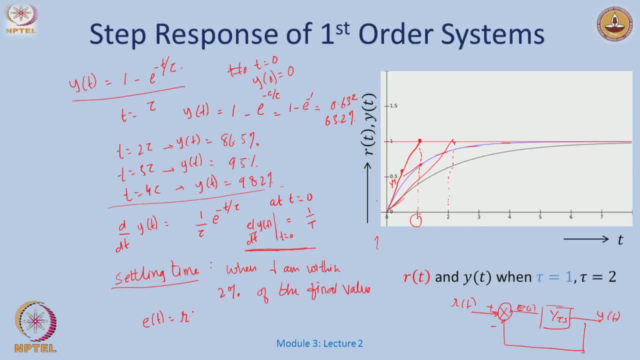 So the error E of t as r of t minus y of t. ok, So what is r of t is just a unit, step 1, and what is y of t? Y of t is 1 minus e power minus t over tau. ok, 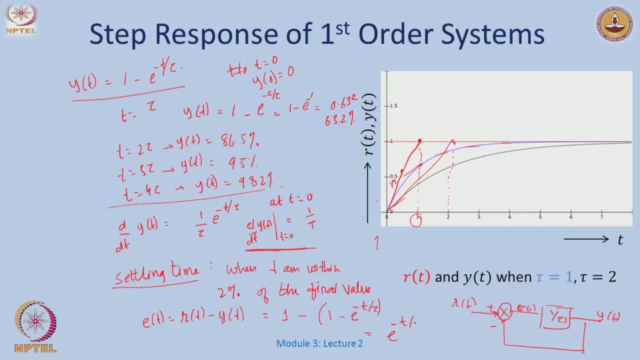 So this is simply e power minus t over tau. Ok, This is all times greater than or equal. to say this is 0 plus ok. Now what happens to error at infinity? right as t goes to infinity. this is just this. is my term right? that it goes to 0 means at infinity. 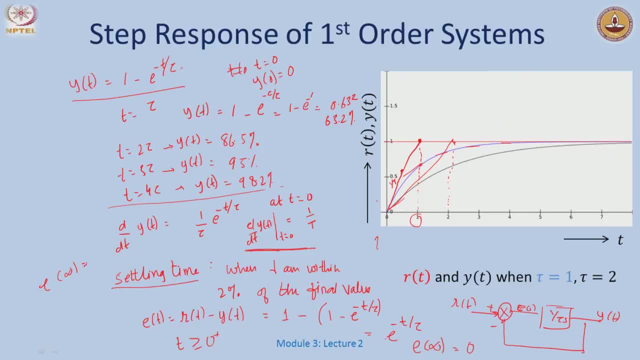 So if E of infinity is 0, from this expression I can say that r at infinity is y at infinity. Ok, And see, this is exactly what is happening here. right at infinity, both signals become the same, right that my system, I can say it is asymptotically tracks a unit step right. 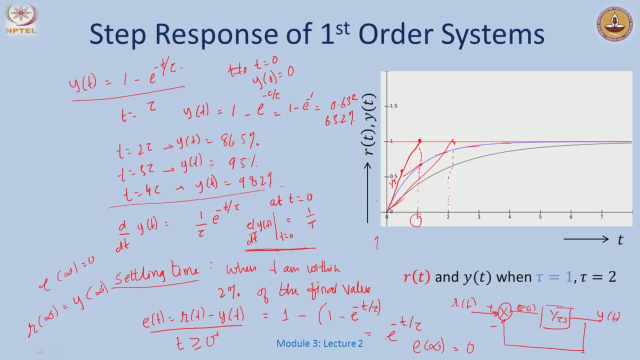 So it is no matter what the value of a time constant is, this guy does a little slower, but it is here. you could have even slower guys which could do here, but they would eventually again go to go to the value 1.. So this system, I would say again: I am sorry defining these terms, but we will elaborate. 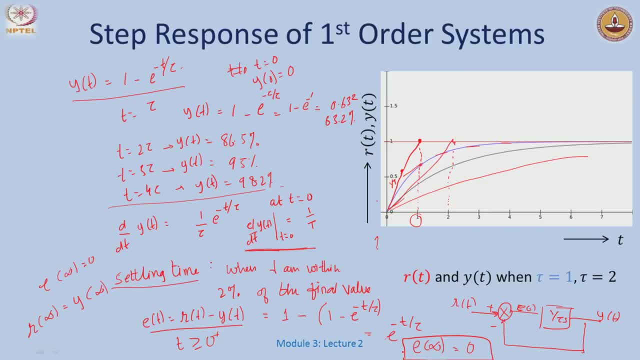 this a little later has a steady state error of 0.. Ok, I can just call this. I am running out of space here, but let me write it here. how do I define this? It is a difference between the reference and the output, and how does it go at infinity? 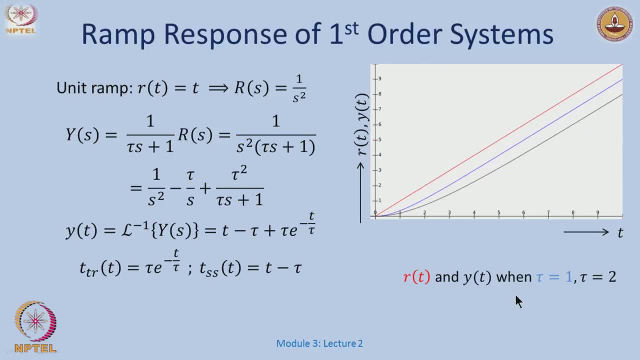 ok. So ok now, what happens when the input is a ramp or when I am actually passing my system to track a ramp? ok, 1 over tau s plus 1 r of s, And then I do this: Ok, Ok, Ok. 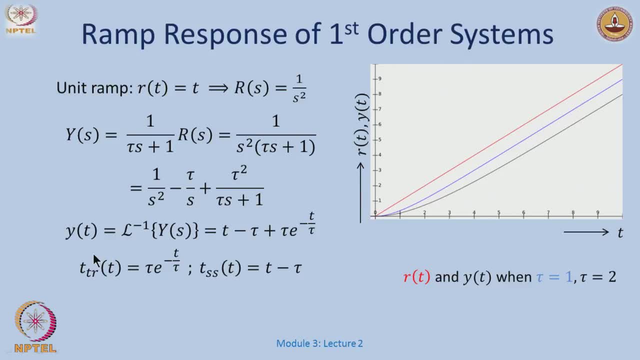 So I do all these things and s? c do the inverse Laplace. the response to a ramp would look like this: t minus tau plus tau e power minus t over tau. ok Again, how do we classify or how do we differentiate between the transient response and the steady? 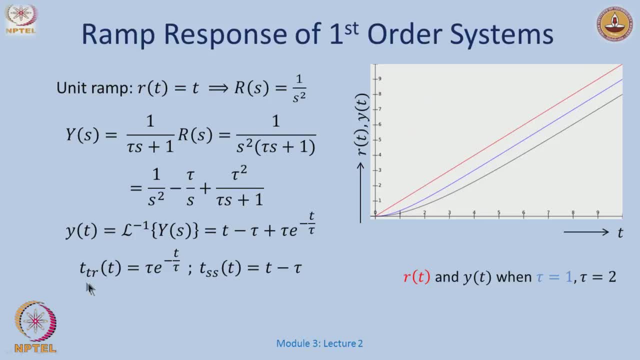 state response. Well, the transient response, well, the one which goes to 0 for very large times, is this guy. and at steady state this guy still remains ok, So it need not be so earlier. we saw in the first example that the steady state was. 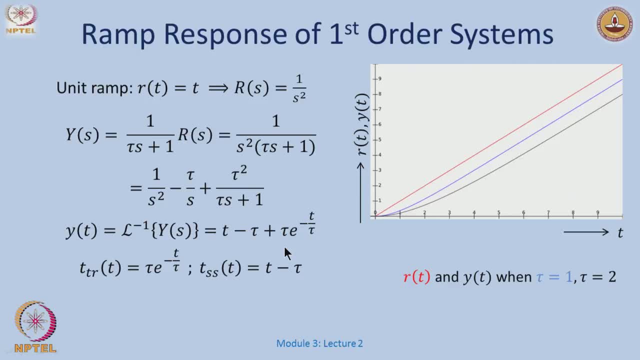 0.. In the second example, when I was tracking a step, the steady state was 1, and now we see it is actually depending on time. also, ok, We will see. is what these things actually mean? ok, So let us see first what is the error? right? 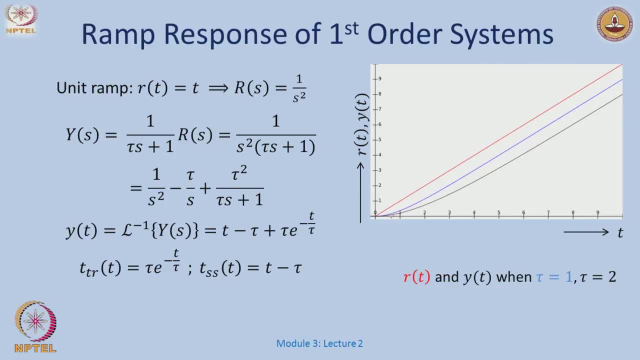 Does at t equal to infinity? are my responses just meeting the original signal or not? right Again, I just draw it for the sake of Ok, Ok, Of completeness here, that here I have r of t, I have 1 over tau s plus a minus and I have 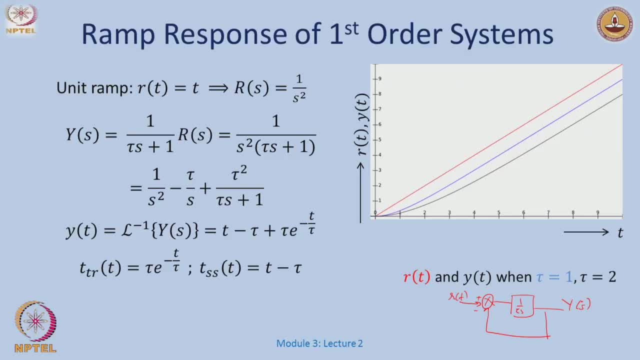 a y of s, So sorry y of t or whatever notation you want to follow. ok, ok, better y of s, because this is s. this also be s capital R of s. ok, So at infinity does my output track the ramp right? So that depends on what is the error signal here. 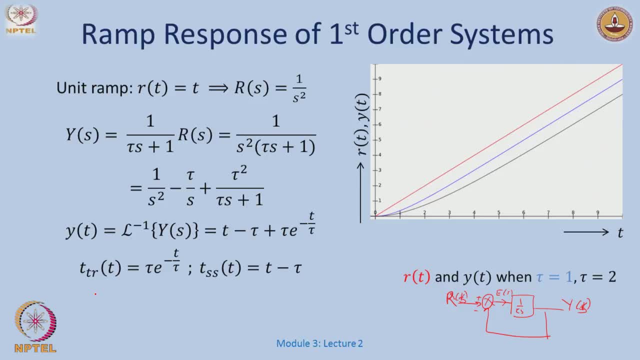 So what is e of s or e of e of t? e of t is r of t, which is my t minus y of t. y of t is the entire thing: t minus tau plus tau e power minus tau over t. ok, So what I am left with is tau plus another tau e power minus t. 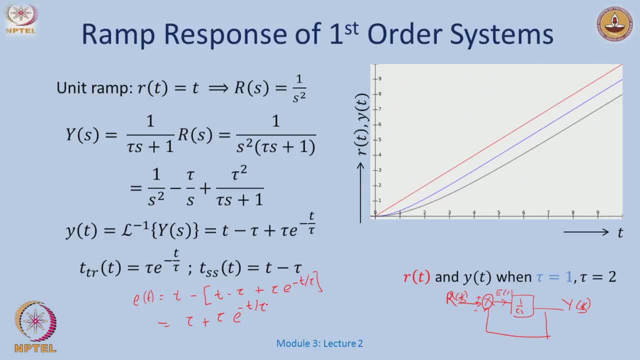 Ok, Now, if I do these things, e at infinity would be well. this, nothing will change here. tau plus this guy at infinity will go to 0. So nothing will be tau plus 0 is tau. ok. Now what does this mean? So this is my r of t, this is my reference signal, right? 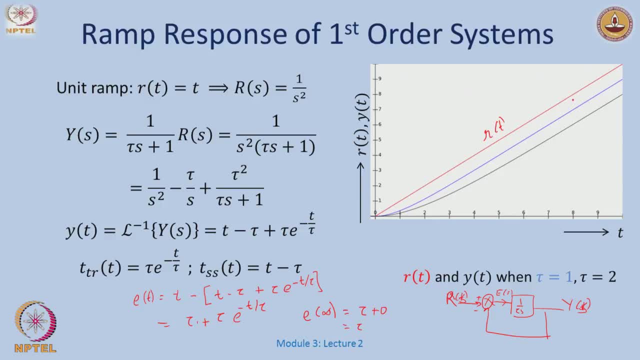 So, as t goes to infinity, I am not touching this guy, but I am actually just at a distance of tau. ok, So I am just at a distance of tau, which is 1 in this case. right here, I am just at a distance. 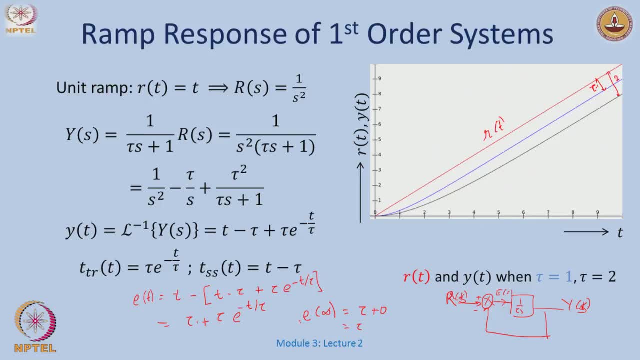 of 2, right. So there is some kind of a steady state error here which is just governed by this number tau. The smaller this number, smaller the steady state error. ok, So what I conclude is that, well, first order system, if it has a ramp, it will have some. 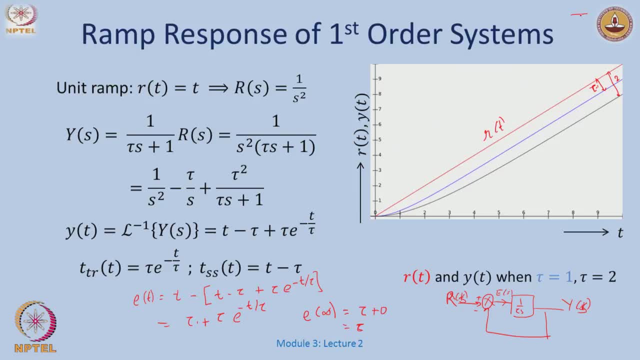 steady state error. ok, How do I encounter the steady state error? Let us say I just again take this example of a pendulum Right And I started with some non-initial condition and I expect it to go to theta equal to 0. if this is theta right, ok, but there could be something in the system we stops it going. 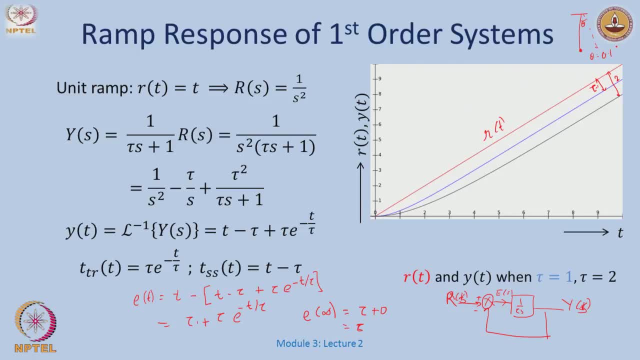 maybe it just stops at theta equal to say 0.1 degrees, right? So that is the idea of this steady state error, right? So it does not really reach the final, the desired value, but some number very close to that. There is an error, but there is a way to determine that error: how small it is, how large it is. 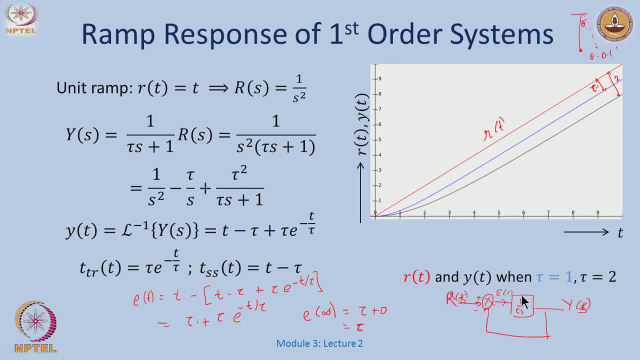 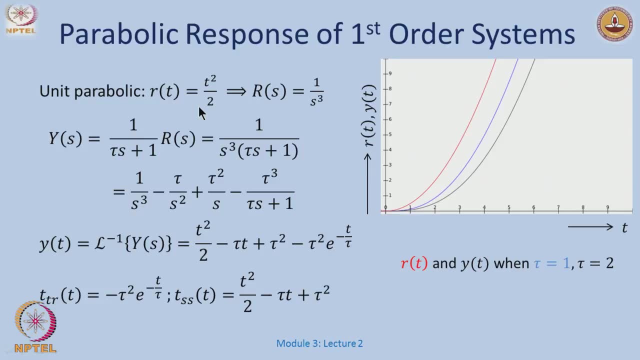 I can directly quantify by just looking at the dynamic Right, Looking at the dynamics of the system. ok, Now, finally, we will see. another test signal is the parabolic input. well, r of t is t square over 2, the, I know, the Laplace transform is 1 over s cube. and I do all these things and 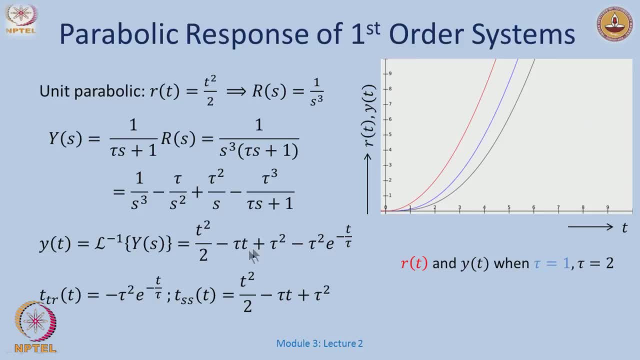 I get signal which is t square over 2, minus these terms, plus tau square and so on. ok, Again, this has a steady state, this transient term which will just die down as time goes to infinity, And the steady state term, well, it is actually looks possibly quite worse right than the. 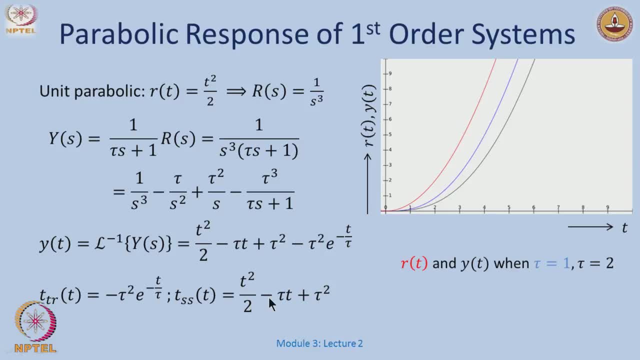 original one. it has a t square term. now, right, this is no longer constant. ok, What does the error do here? right? So can my system track a unit parabola? ok, So the error e of t is my reference signal, that is t square over 2, minus the output that. 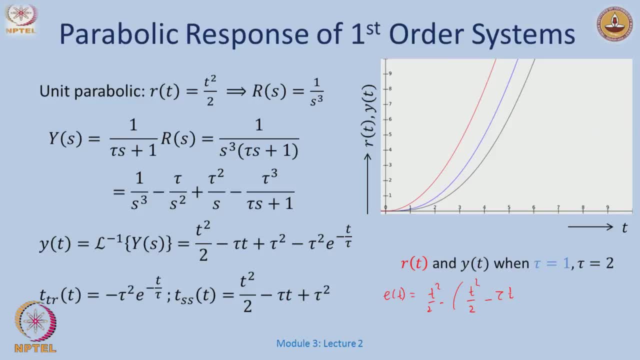 is t square over 2 minus tau. t plus tau square. ok, I would exclude this exponential term Ok, Because I know it will not contribute to the steady state error and we will go to 0 anyways. So this will be tau of t plus or with a minus tau square. 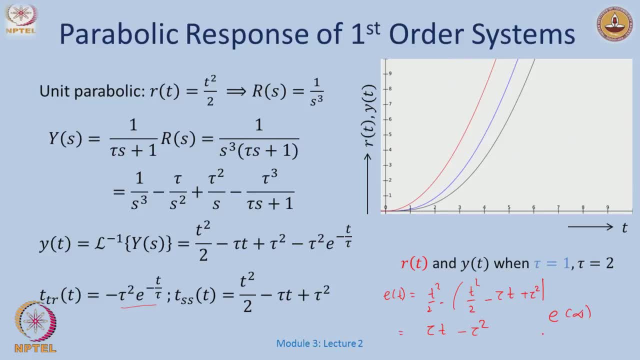 So e of infinity is actually a little strange here, right e when t goes to infinity, this guy also goes to infinity, ok, So the error will be very large. So if you see that the distance between these two, this is my actual reference signal and 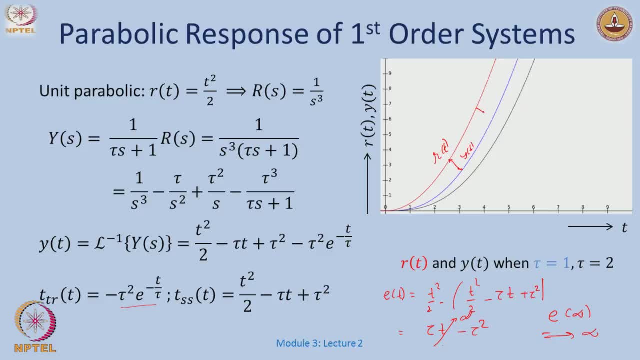 this is my y of t. So as I go to infinity, this distance will keep on increasing right, So it will keep on increasing, increasing, and then, if you keep plotting this forever, you will see that, you know, distance actually becomes unbounded. similarly with here, with 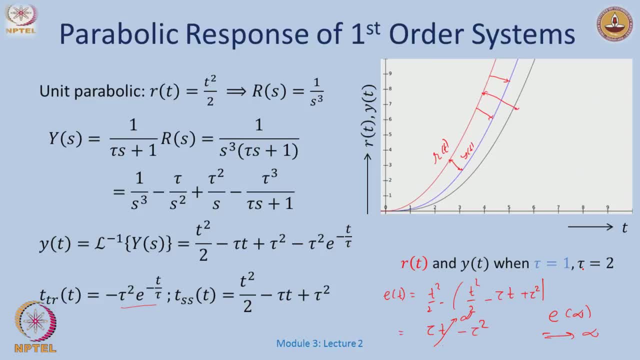 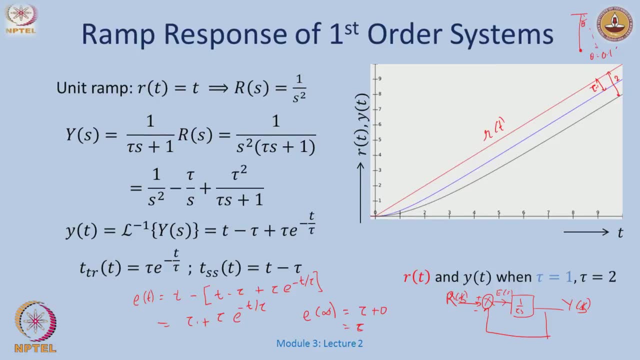 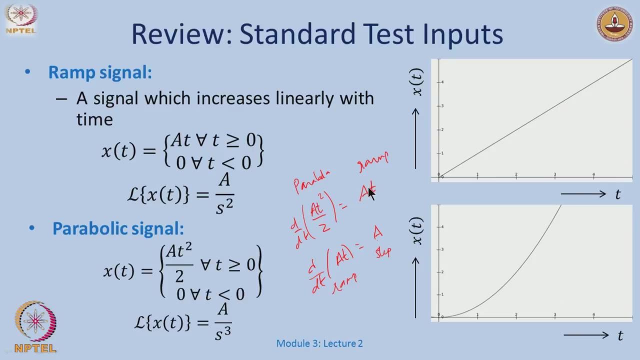 a different time constant of tau equal to 2 right. ok, Before this right. So when in one of my- you know- earlier slides, what I had shown was that this things right, I take a parabola, I differentiate it, I get a ramp. 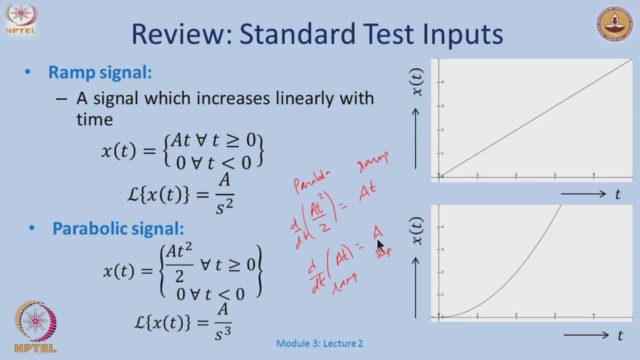 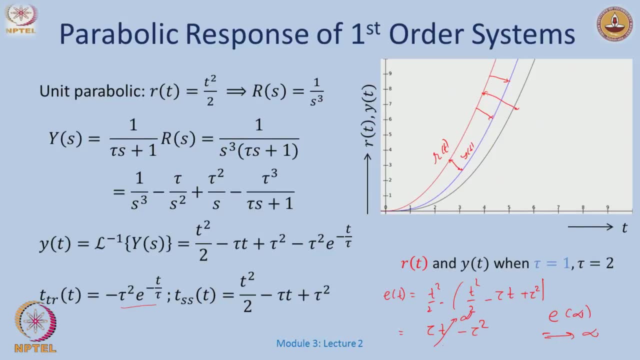 I take a ramp, I differentiate and I get a step. Now let us see if the responses also follow some kind of a pattern like that. ok, So this is my response here, right? So this is this entire thing or this is this guy? ok, 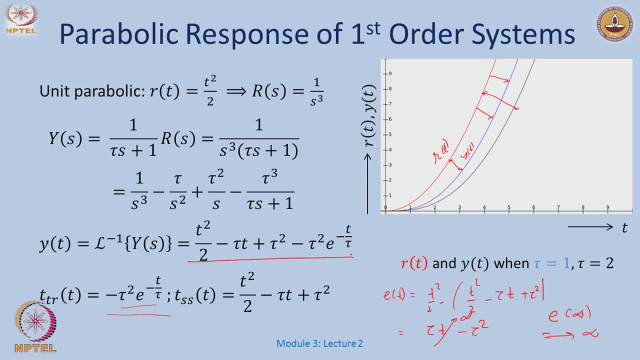 So just let us differentiate this with time. So d over dt of y Right, d over dt of y, t in this case would be t minus tau, and then here you will have plus e power minus t over tau. 1 over tau will be here something like this: ok, 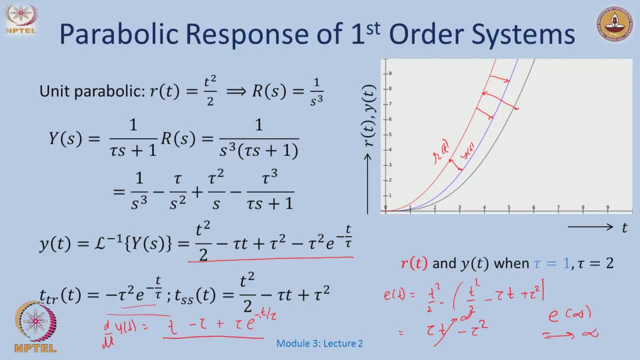 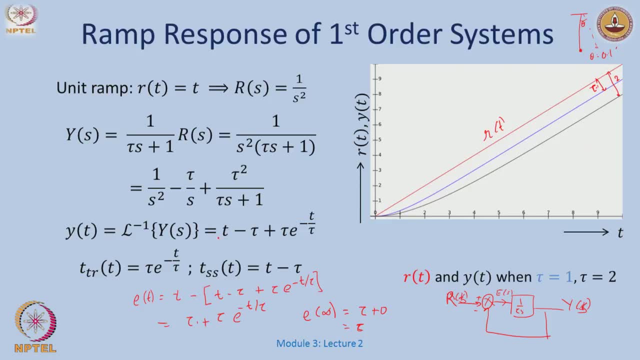 Now just remember this: t minus tau plus tau, e power minus t over tau and this looks something like this: Right, Exactly this one, right? This is just the differentiation of dy by dt for a unit parabola. ok, So I differentiate the response. I get now the response to a unit ramp. ok. 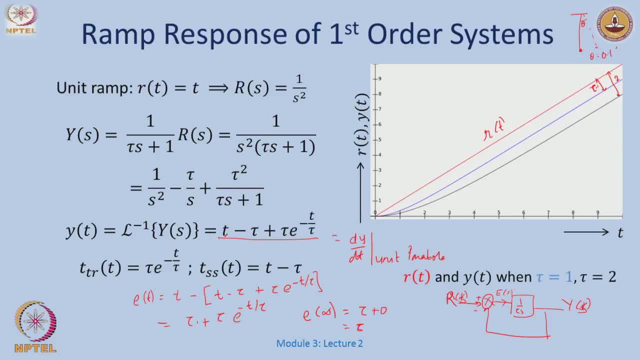 So the differentiation holds until now. ok, Now let me differentiate this again: dy by dt, dy by dt. When the input is Right, Right, This ramp is: this will be 1, this will go to 0. this will be a minus e power minus t over. 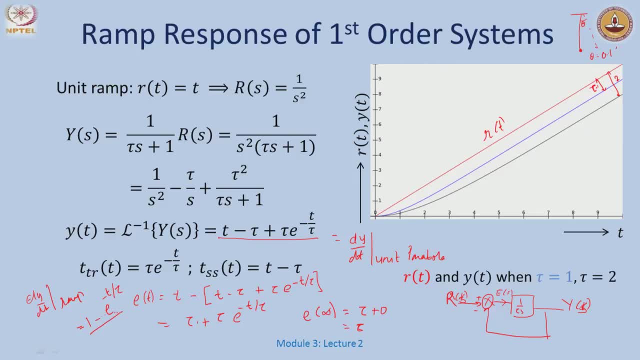 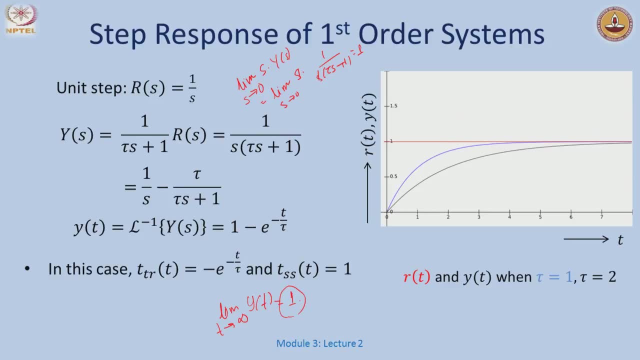 tau. ok. Now just see how this looks: a 1 minus e, power minus t over tau go back, slides. and this is the same right, this one, ok, And I can keep doing this right. So you see that if the signals are preserved under differentiation in this way that I differentiate, 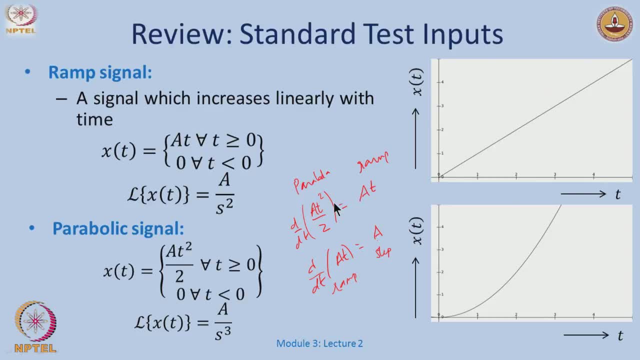 a parabola to get a ramp. the responses are also follow the same pattern. If I know the response to a parabolic input, how do I find the response to a ramp? I just differentiate this Again. from here to here- one more differentiation. here to here- one more differentiation. ok, 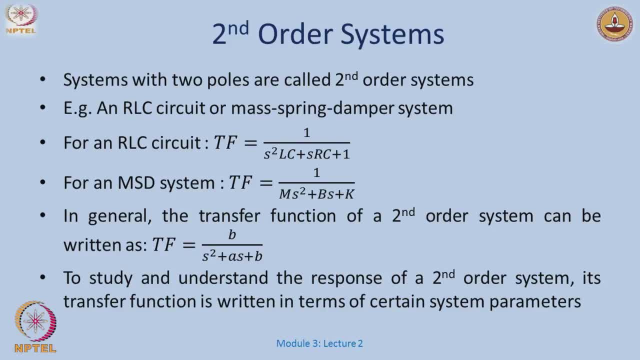 Good, Now we go to something slightly complicated, but still not very complicated, but very useful. So second order systems: these are the systems which have two poles. ok, We have done lots of examples on this. had a typical RLC circuit would have a transfer. 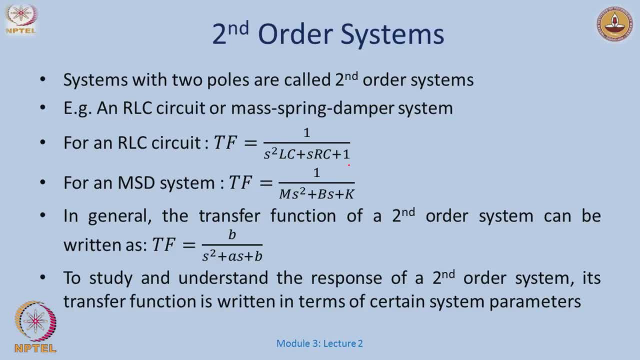 function like this. If you remember vaguely, this was a transfer function between the voltage of the capacitor and the input voltage. Similarly, for the mass spring damper system where I was taking the, you know the input was a force, output was a position or a velocity, one of those. and then in general I can write. 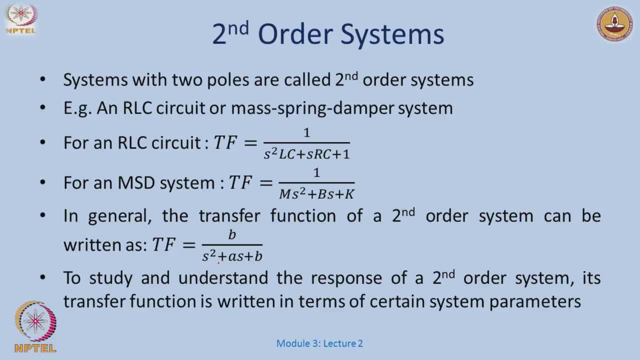 transfer function as well. a second order: polynomial in the denominator and some number in the numerator, and I will, slowly, we will learn why these are equal, what are these numbers, and so on. right, ok, So the response here will be a little more tricky than what we saw earlier. ok, 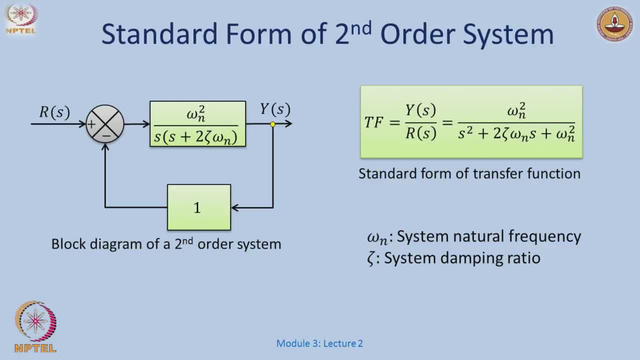 So how do I derive the system? ok, let us me start with a open loop thing which looks like this: I have a unity feedback and I go to a closed loop transfer function which looks like this: ok, Some terminology which will shortly be clear is that omega n is what I call as the natural 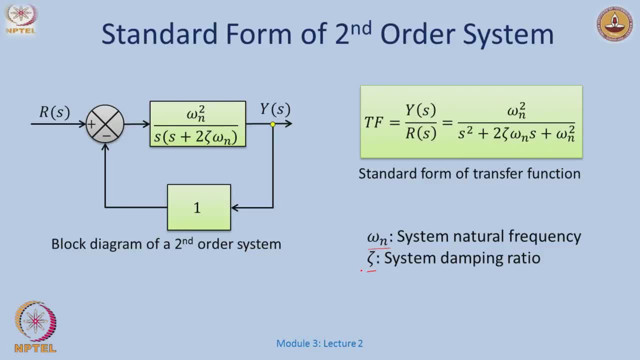 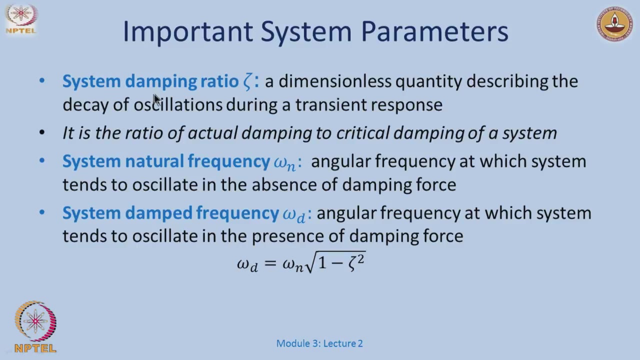 frequency of the system. zeta is a system damping ratio. ok, Let us just remember it with this names at the moment and we will see slowly what they could mean. ok, Just some properties of it. the damping ratio is a dimensionless quantity and it describes. 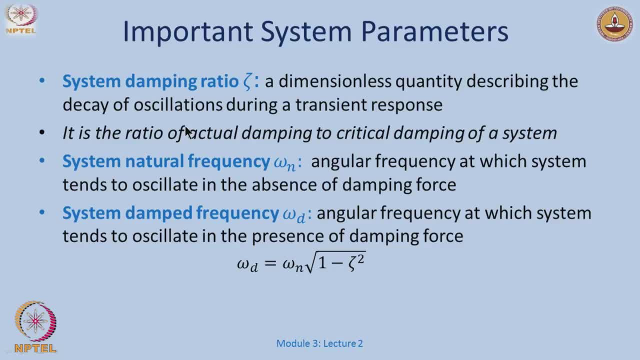 some kind of damped oscillation during the transient response of a system. ok, So this we will leave to the next lecture or the lecture after that. that is, it is a ratio of the actual damping to critical damping. no need to understand this statement at the 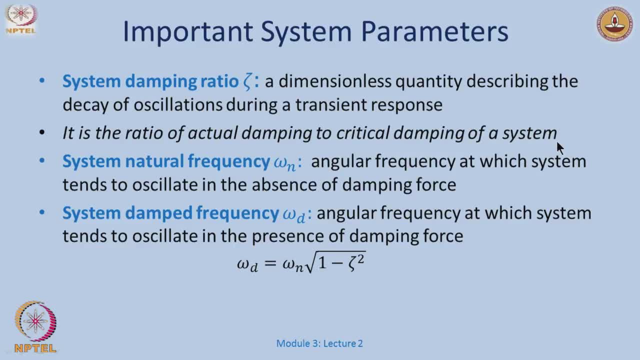 moment, but we will recollect this when we go, and then you know. try to justify what this means. So is the frequency at which the system tends to oscillate in absence of a damping force. ok, this will be clear shortly again, together with omega d, which is the damped frequency. 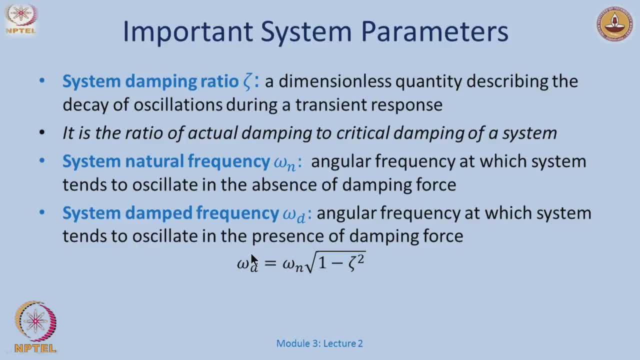 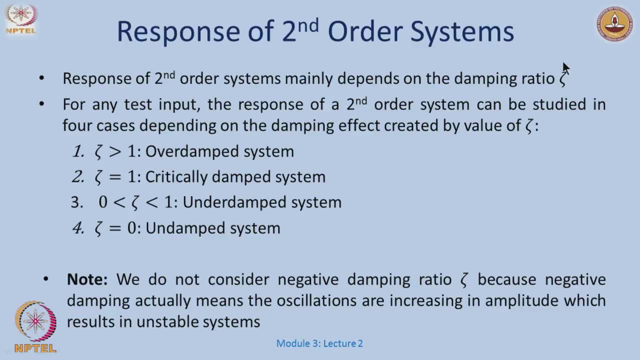 of the system? ok, So will. I can come back to this as we learn it through some examples. So the response is essentially now depending on the damping ratio. zeta- some classifications before we understand them physically is ok. Question: when zeta is greater than 1, I called my system to be over damped. zeta is 1. it is a critically. 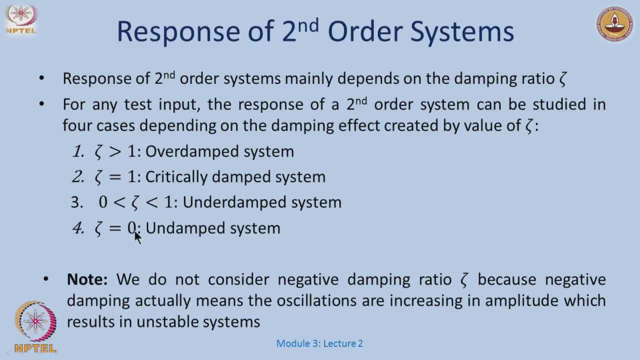 damped zeta between 0 to 1 under damped zeta equal to 0. undamped systems. You might have encountered these words somewhere earlier in some of the courses. if not, do not worry, we will try to define all those things And of course we are not really interested in. 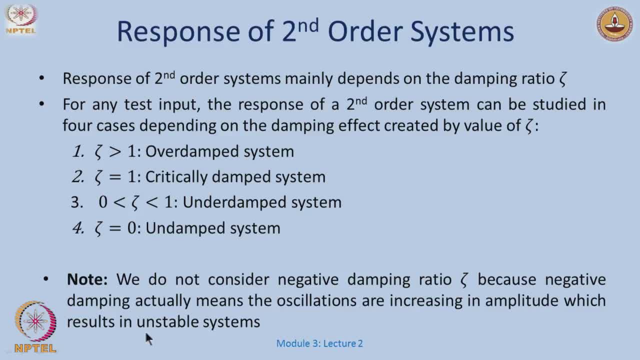 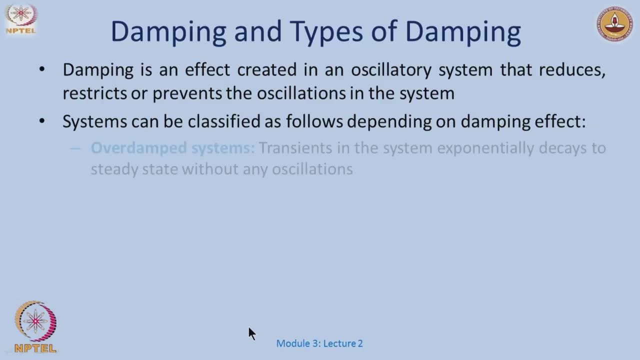 negative damping at the moment because, again, all the things we are doing are restricted to stable systems. but, you know, a system with a negative damping ratio could resemble a behavior of an unstable system which we are not interested in at the moment. ok, What is a damping right? So damping is something which kind of reduces or prevents oscillations. 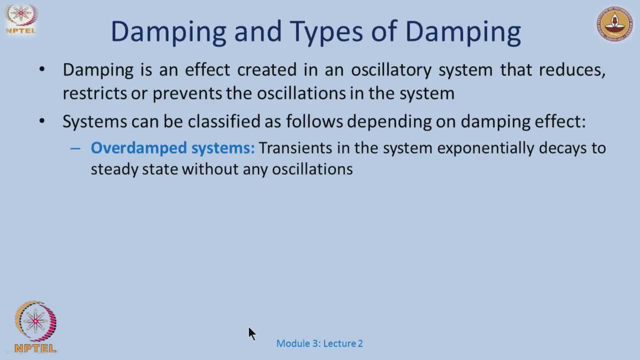 in the systems right. So I could have systems which are over damped in a way that transients exponentially decay without any oscillations. I would have critically damped where you know the system is over damped. So I could have systems which are over damped in a way that 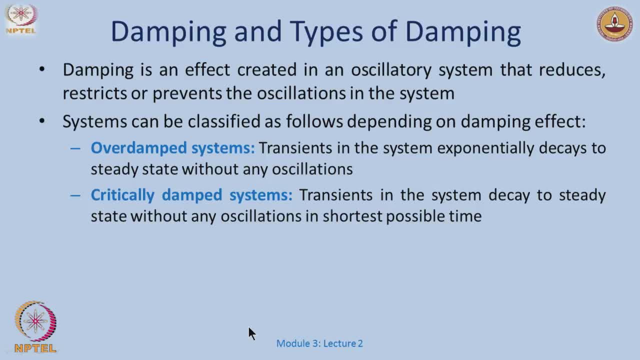 transients exponentially decay without any oscillations. So I could have systems which are over damped, where you know the systems decay to the steady state value with or in the shortest possible time. I could have oscillations which actually go to 0 and I could have undamped. 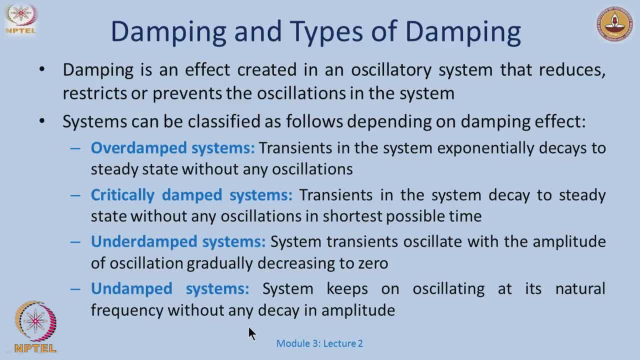 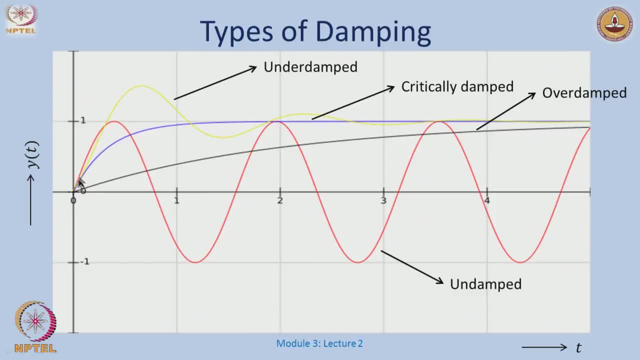 systems, systems which just keep oscillating at its natural frequency without any decay in amplitude. ok, So a typical response, the red color here would be an undamped system. ok, So let me see if I can see the red color here. 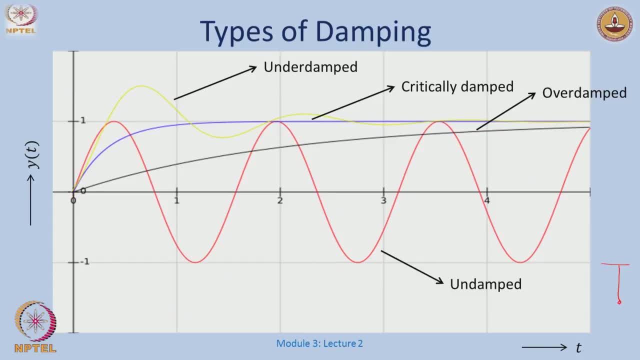 I could explain you with simple pendulum example. right, So I am. I am here, this is my theta equal to 0 position and say I have an initial condition starting at, say, theta equal to some 15 degrees, whatever some other theta, right I am starting here- if the system does not. 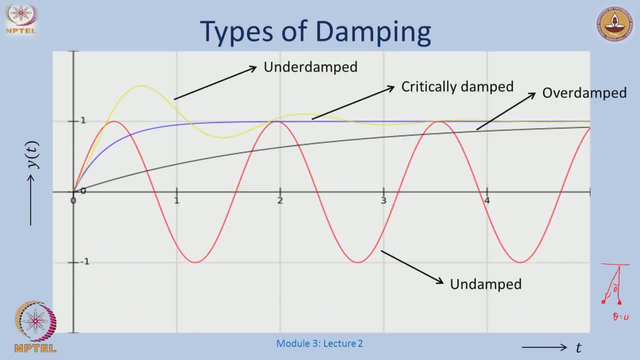 have. it is not subject to any sort of friction, either here or in the air. So what will be we expect is it just keeps oscillating, right? So you just go from theta equal to 15 degrees. So this is a plus. if this is minus 15, it will go to plus 15 and just keep on doing. 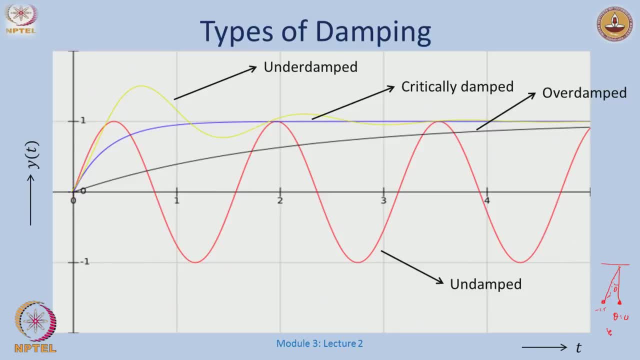 this right. So this will correspond to the behavior when theta is 0, and I will explain you this mathematically very shortly. There could be cases when I could have a situation where this guy is goes from 15, maybe it will go to a 14.9 here. come back and it will keep. 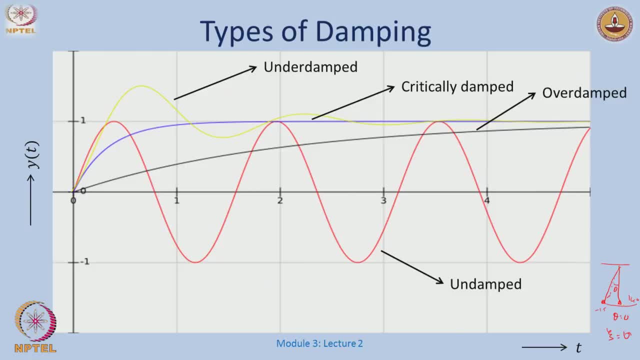 on, you know, oscillating, go back and forth, back and forth until it returns to 0. So it reaches this point. So these are called under damped systems, right when theta was less than 1. There could be a situation where I start from theta equal to 15, I go and I 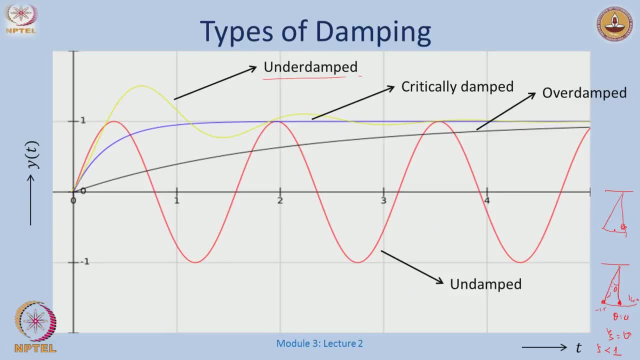 just slowly settle here. I do not go to the other side, I just go and I just stop here. ok, There could be say like this is some time, say in 1 second. There could be situations where I start from here again and I go very slowly and say I am going in 3 seconds There. 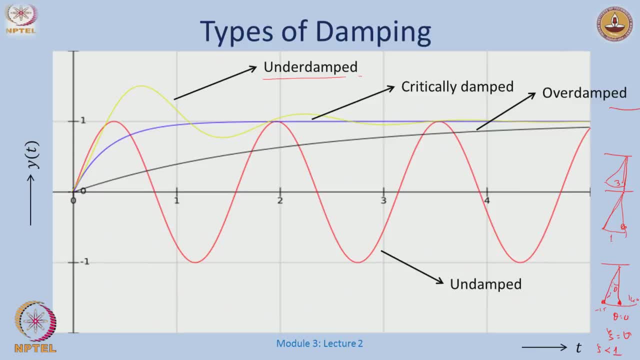 could be even worse situations. So I am not going, I am not crossing this line. I am not crossing this line. the luxman Rekha here, So you can call it. There could also be situations where I start at theta is again 15 or minus 15, depending on the convention that I am going. 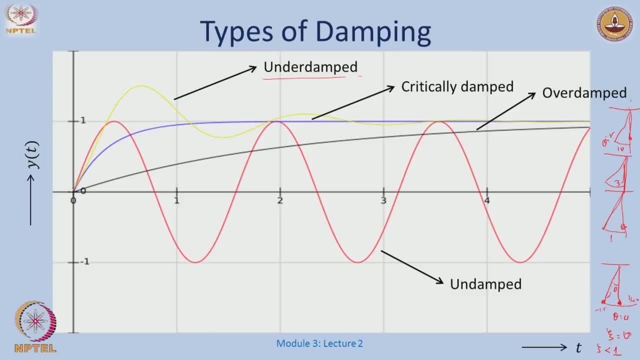 very slow, very slow, and I just stop here. it could take me 10 seconds, ok, So few kinds of responses. zeta equal to 0: I keep on oscillating right For some value of zeta less than 1: I am oscillating. 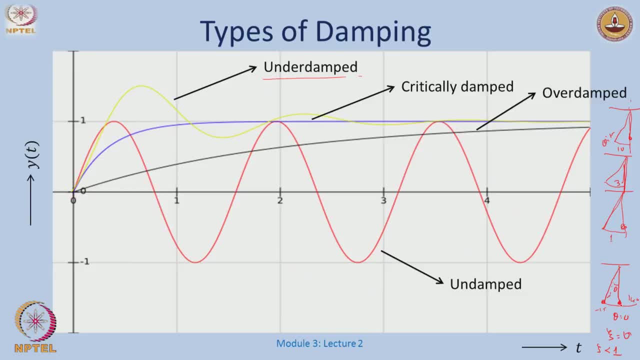 but my oscillations are dying down, dying out. before I reach this steady state position, There could be situation where I just go from here till here in 1 second and just stop. I do not go beyond theta equal to 0, it could take 3 seconds. it could take 5 seconds. So 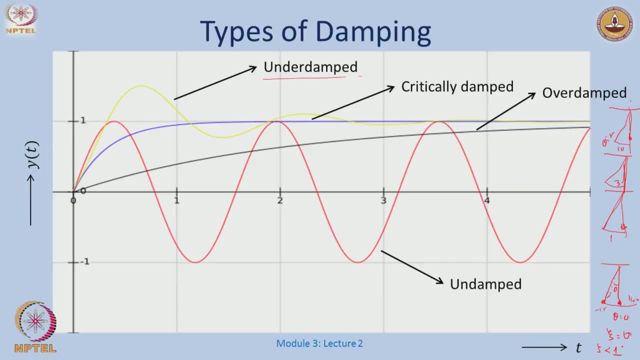 the fastest value of- and these things will vary with zeta right, zeta equal to 0, zeta less than 1, and then all these behavior would be zeta greater than or equal to 1.. So the fastest where I can reach here and stay is the critically damped response ok, which is 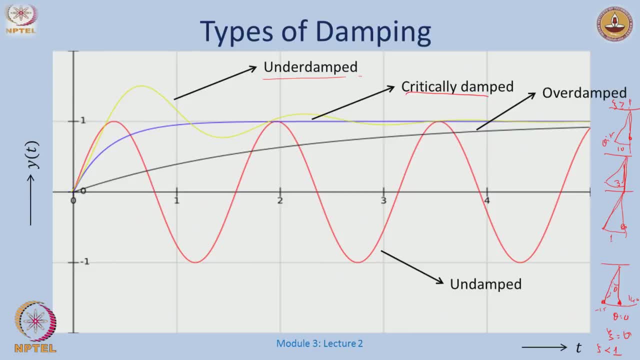 like the blue line here And for damping anything larger than that. I will just keep taking a longer time. I could have a response also here, right, some something like here which could be say, zeta, still there. So these are typically the 4 kinds of responses which we will encounter in designing a system. 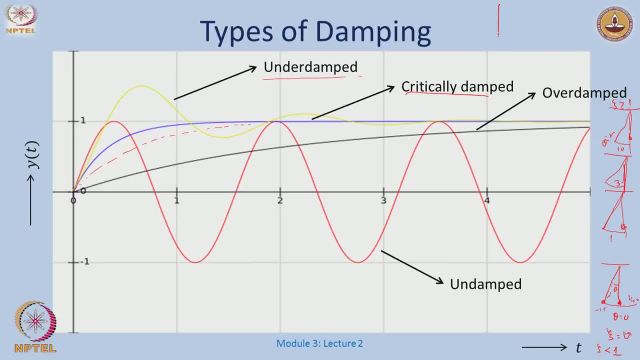 If I take, for example: I want to design a lift or an elevator and I want to go from say this is level 1 to say level 2.. I am lazy and I do not want to walk and I take this elevator And I go up. I do not want my system to go to 2,, 2 point. you know, half way to the. 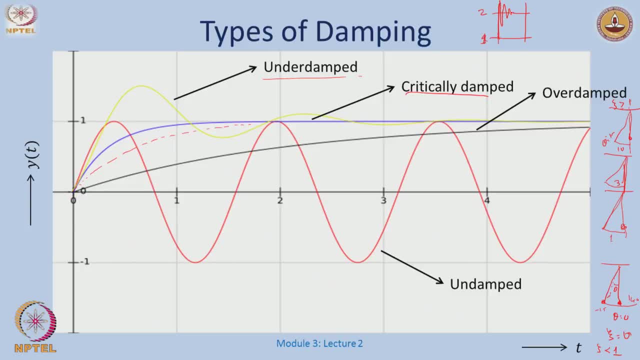 third floor. So I will go back here and then do this, and I do not want it to do this right now. that will be very unpleasant, right? Even if you know, like you see in the TV, even if the pickup water cone is stuck with me, this is still be very unpleasant And therefore what we 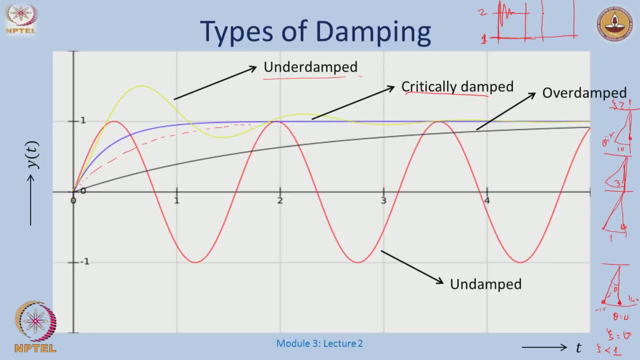 design this systems are to be critically damped or like slightly over damped. right that I just go here and I just slowly settle down here, right? So again, depending on my requirement, I would just want to, you know, have my system to go. So I would just go here and I just 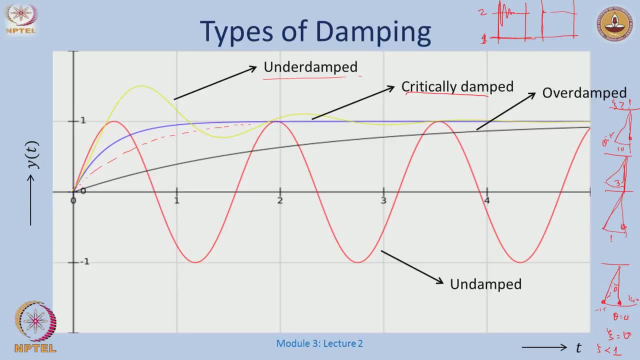 slowly settle down here, right? So again, depending on my requirement, I would just want to know how my system behave as this is going on. So I did not want to be either be underdamped, critically damped, or even sometimes over damped. ok, 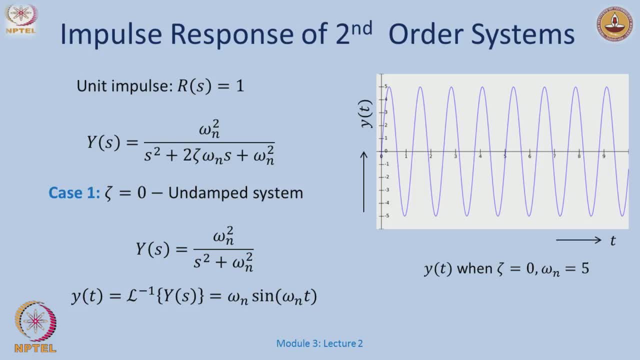 We will characterize all these very shortly. ok, So how does my system behave, again, with the standard test signals? So here I have to be careful that there is another thing. this is not just a test signal, but something depends also on the value of zeta, right? So 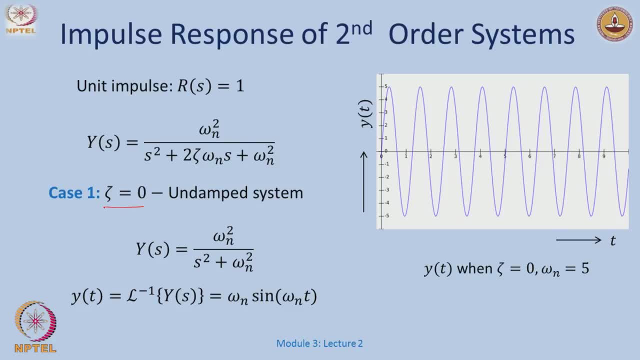 earlier my formulas were easy to remember. but here you know, the zeta adds more complexity to me, right, or more. it presents me with more test cases. So y of s is omega n square, s square plus 2 zeta, omega n? s plus omega n square. ok, So 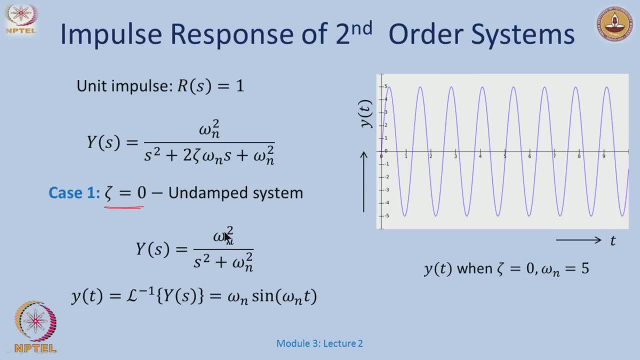 zeta equal to 0 would be. this guy would go away. y of s is this one, and I can do the inverse Laplace and I can just say that I just have a sinusoid of some frequency. omega n- ok, Let us just highlight this very nicely. omega n- ok. How does the response look like? Well, 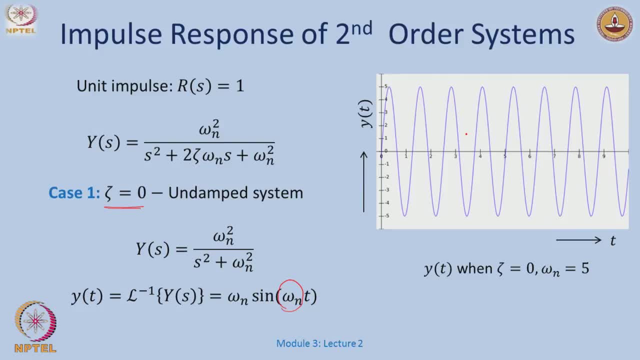 the response is just a sinusoid. I say: what is its amplitude? Well, amplitude is this one, it could, ok. Now what I am interested is the frequency. ok, Zeta is 0 and if there is no damping it will oscillate at omega n. ok, and therefore, 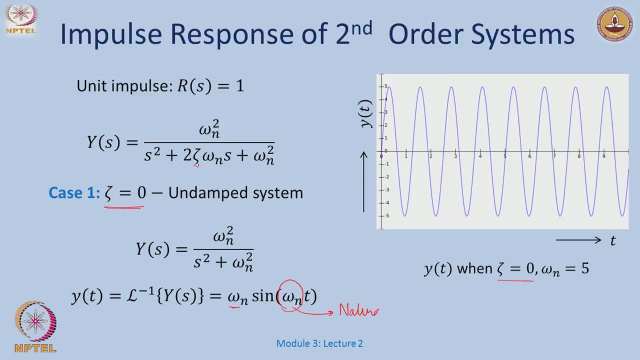 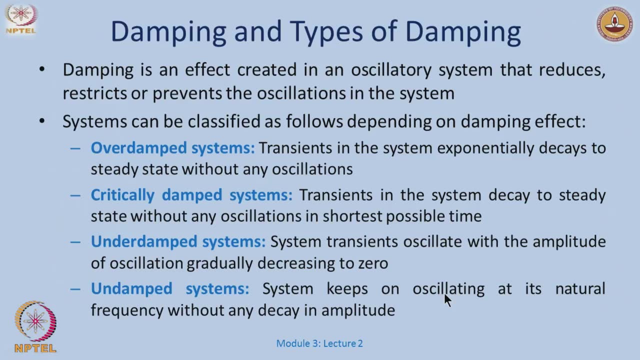 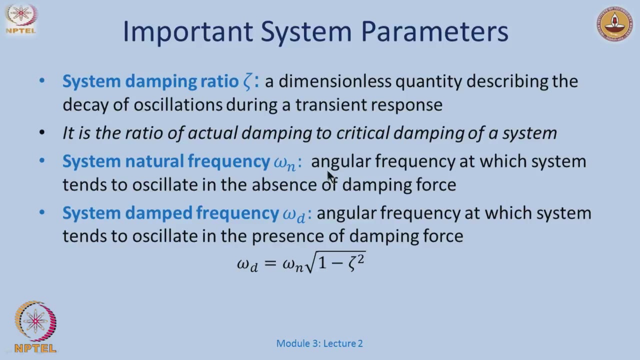 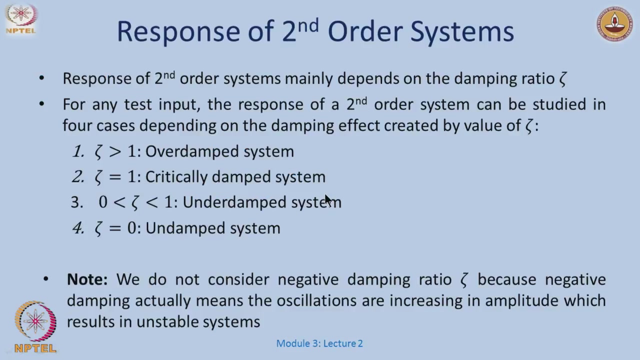 I call this as the natural frequency as defined earlier. right, So here. so, for example, I did. we define that: yeah, this the system: natural frequency, the angular frequency at which the system tends to oscillate in the absence of damping force. that is exactly what we did. 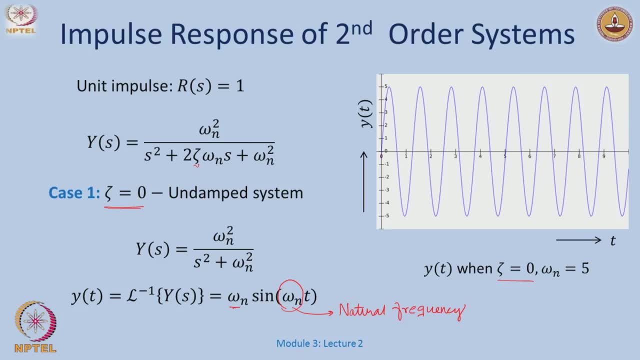 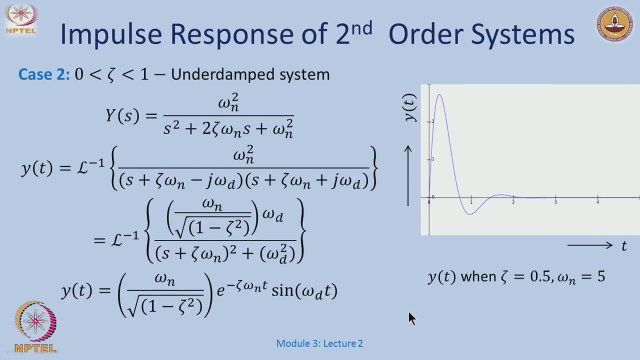 now There is no damping force, zeta disappears and then my naturally my system just oscillates. ok, So this is the natural frequency when there is no damping. ok, So let us, Let us make things a little complicated, ok, So sigma between 0 and 1. ok, So, before I, 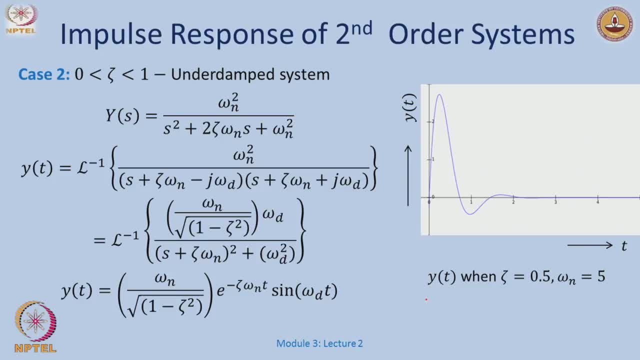 do this. I will just do some very short calculation here. So look at the denominator. I have s square plus 2 zeta omega n. s plus omega n- square. ok, So just to say I know, if I look at you know how do I find the roots of this? These roots would be ok. So minus zeta omega. 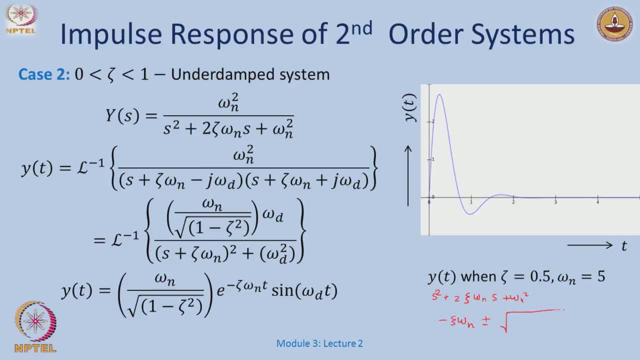 n, zeta, omega n, square, and then we divide by 2 and you know it is on the standard formula. Now this is minus zeta omega n, plus minus omega n, square root of zeta square minus 1. ok, Ok, Ok. 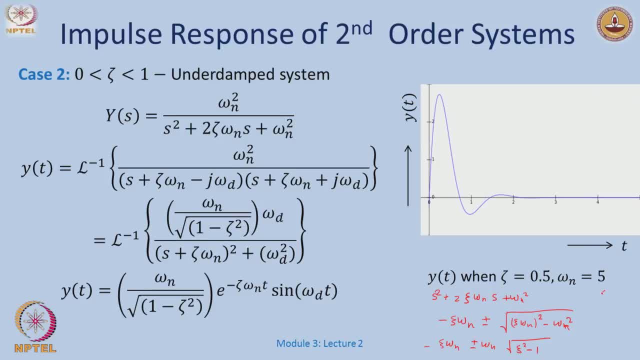 No, thank you. Now, when zeta is less than 1 and of course greater than 0, this will become a complex number, right? and therefore the roots will look something like this: let us say here- and I call this guy ok, So if it is complex, I will just ok, I will just write it here: minus. 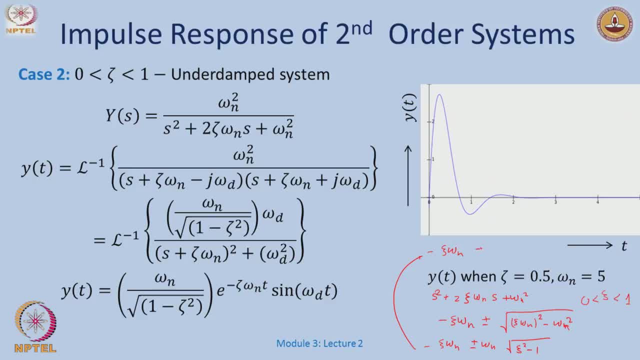 zeta omega n plus minus j omega n, square root of 1 minus zeta square, and this guy I will call as omega d. ok, So, and this is how this roots now expanded: this s plus zeta omega n, minus j omega d and plus j omega d. exactly what is here? ok, Now. 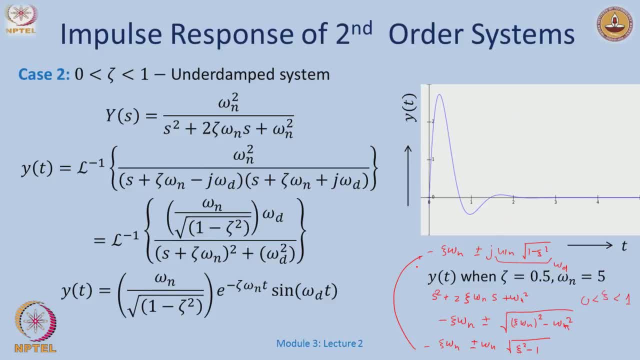 the. I just want to see the natural response, or the impulse response, And I see, I just do all the Laplace transforms, inverse Laplace transforms, which I learnt earlier. I see that y of t is some number here, omega n, blah, blah, blah. then I have an. 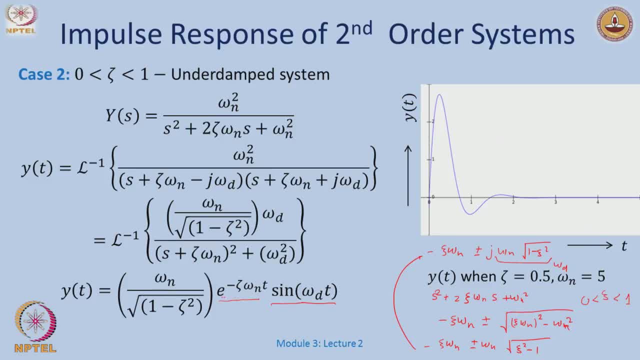 exponentially decaying term and this guy. I say exponentially decaying because all these guys are positive and with time, you know, it just falls in value and goes to 0. ok, It is still now. earlier here I had sin omega n t, whereas here now I still have a sin omega. 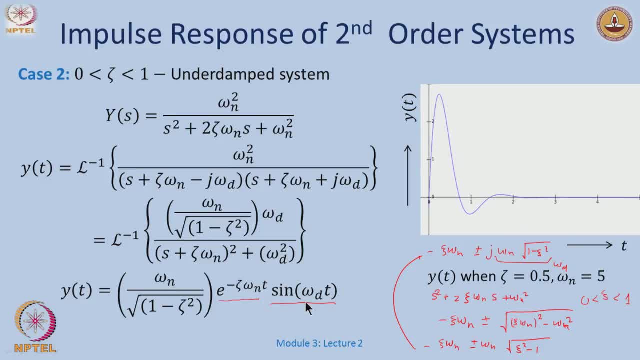 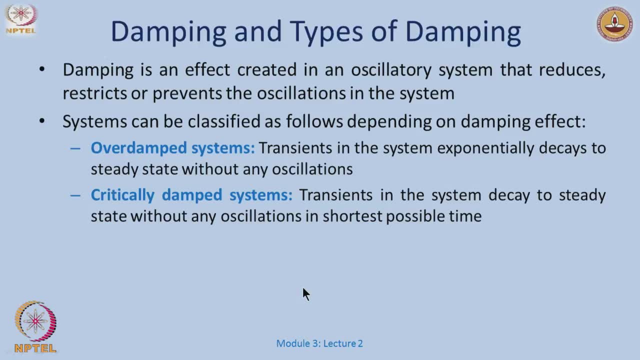 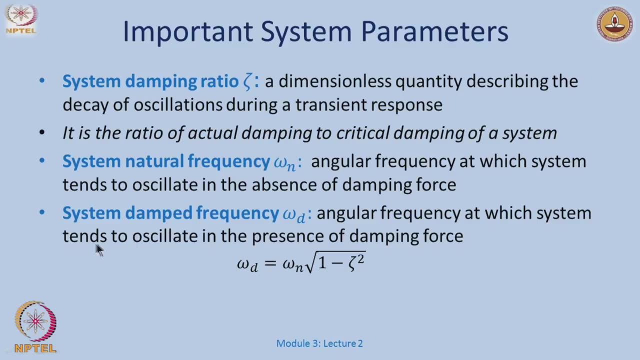 n sin curve or a sin wave, but with a different frequency. that is, omega d right, And therefore I call this as the damped frequency, the system damped frequency, angular frequency at which the system tends to oscillate in the presence of a damping force, and zeta was greater than. 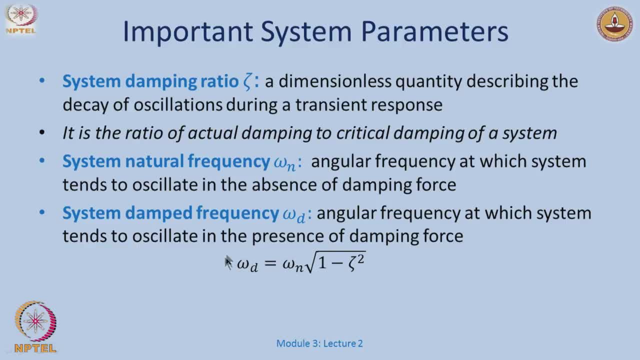 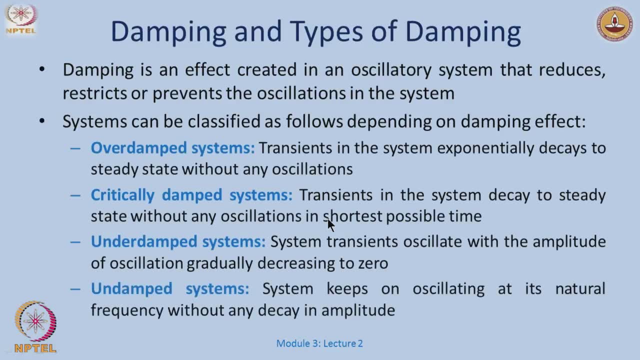 0, but less than 1, and this exactly the formula we use there. And this is omega d is not because of any magic that I define It, just because it just sits in beautifully here in the term of sin, omega d, t, right This: 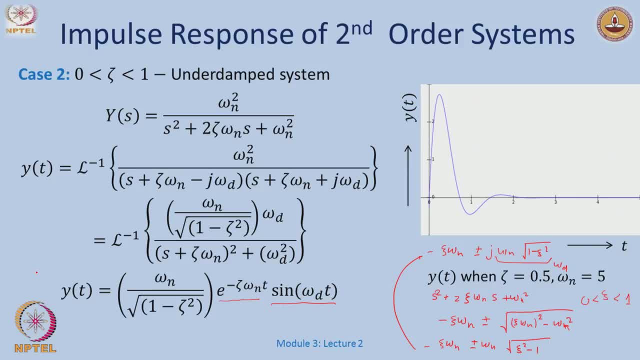 is why I call this omega d t as the damped natural frequency. this is omega n: square root of 1 minus zeta square. ok, So this is the damped frequency and, of course, I have this exponentially decaying term And if you see the response, where it will? it will keep oscillating. 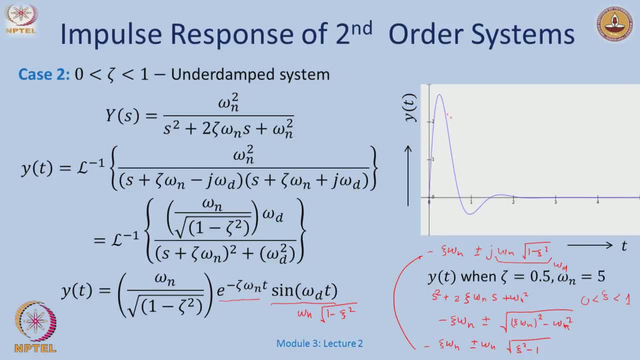 and eventually go to 0. that is the response of the pendulum which we are talking about. right, when zeta was greater than 0, but less than 1. right, and this is the sign here says that will there will actually be oscillations. right, I will just go to whatever this number. 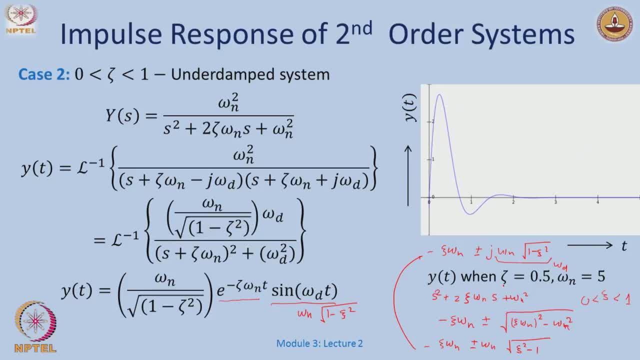 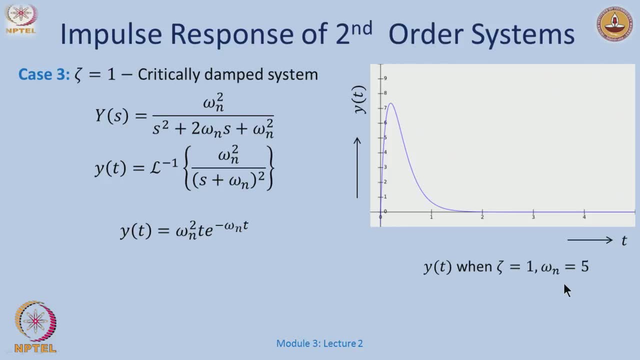 here is: come back and of course, this numbers and depend on what are the specific values of zeta and omega n? ok, Now other case could be when zeta is 1.. So when I, when zeta is 1, my expression for y: 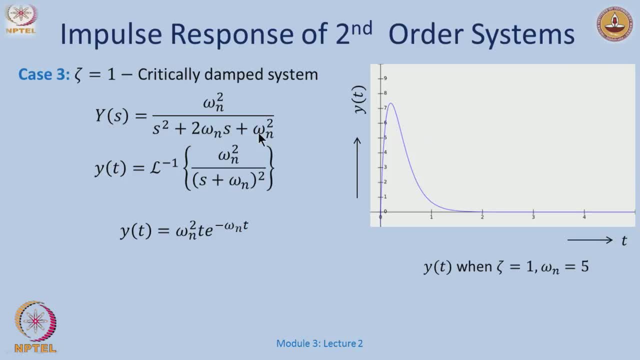 just looks like this: S square plus 2.. 2 omega n s plus omega n square and the inverse Laplace would just be like this: right, And if you see that the sinusoidal term has disappeared, which means there will not be any oscillations. 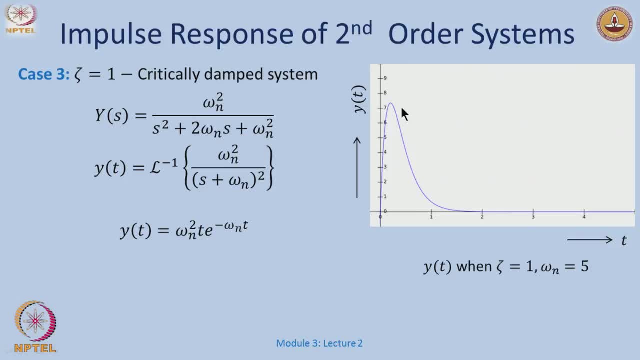 However, you will see that as time goes to infinity, I just come back to 0. ok, This is again for a particular value of zeta equal to 1 and omega n. will we later investigate what happens for larger values of zeta and so on? right, So this is so here for a system. 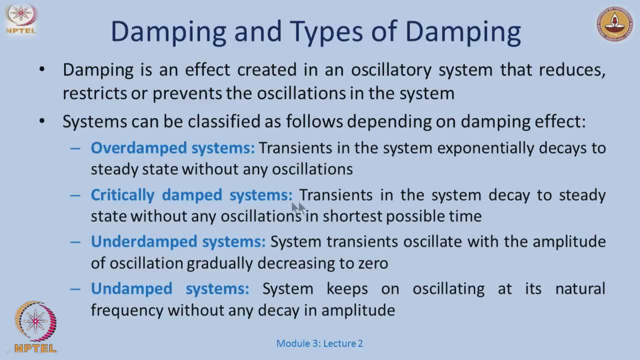 which we actually called Now as a critically damped system. the transients in the system decay to a steady state without any oscillations and in the shortest time possible, right as we had defined in the case of the pendulum. here, This is the shortest time and this is a critically damped case. 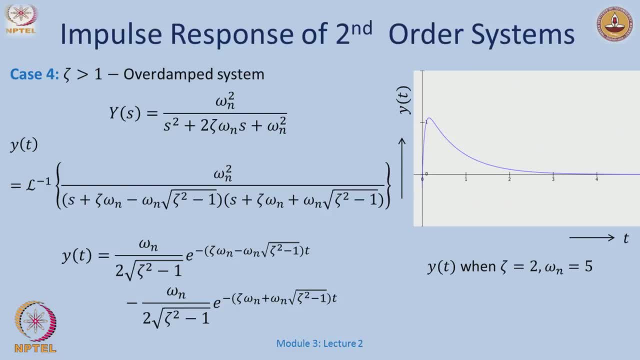 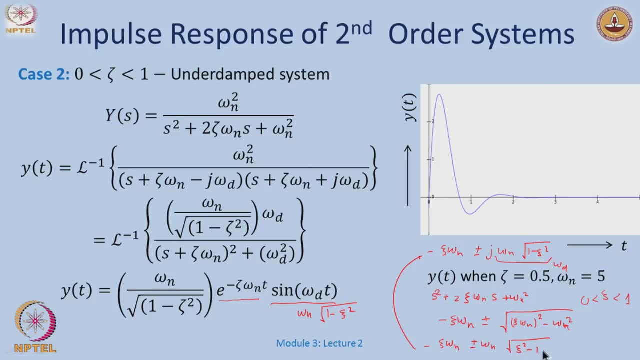 ok, Now I could go to over damped system where this zeta is greater than 1, in which case these roots will just be real. right So, zeta less than 1. I had complex roots, but I will just have real roots. right So, zeta less than 1. I had complex roots, but 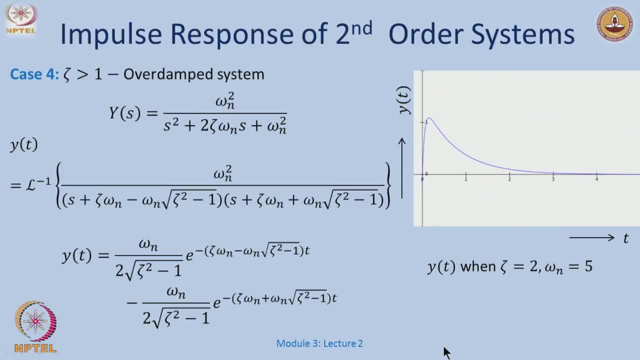 I will just have real roots, right. So zeta less than 1. I had complex roots, but I will just have real roots, basically ok. So what happens here? So omega n square plus s square, 2, zeta omega and S omega n square: I can just write it as a composition of 2 real roots. 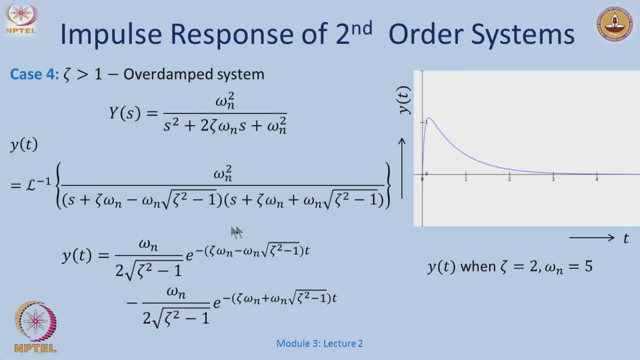 like this, for which the response looks like 2 exponentially decaying signals: right zeta omega n- blah blah blah and zeta omega n- blah blah. and again this response. we could see that there is no oscillating term, there is no sinusoidal term, So we just go the here. and then just have it here by putting endeavor right to n. Why is it a sinusoidal term right? There is no sinusoidal term here too, So it is only continuous. replace with zeta n plus a minus spirit. Now, whatever the situation is, say whether 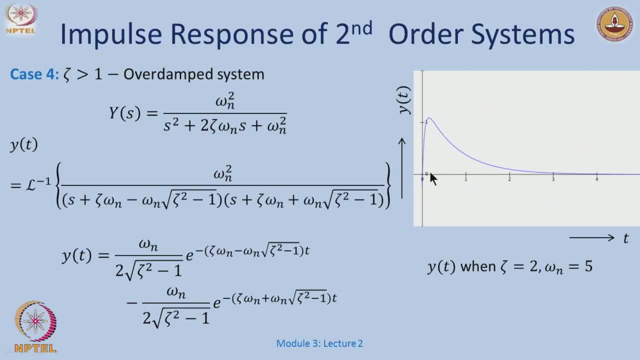 the 2 integration. is there right or not For the解 transformation that we have done? this is also very simple. just come back, Possibly when zeta equal to you know. 3, you might have even much slower response like it could- sorry, it could take even much larger time like this and so on. 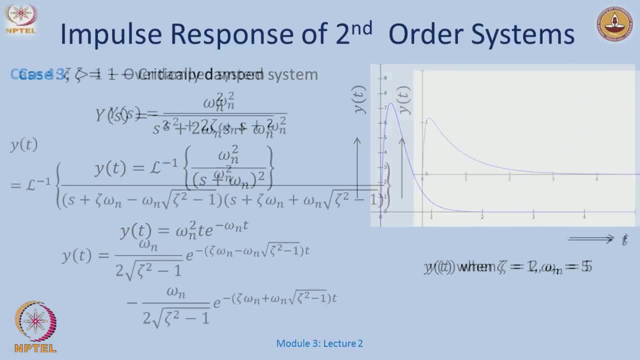 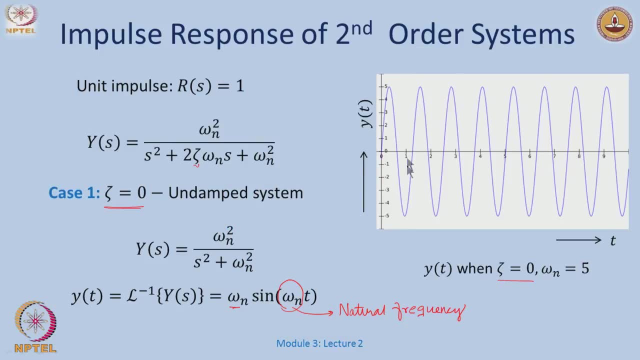 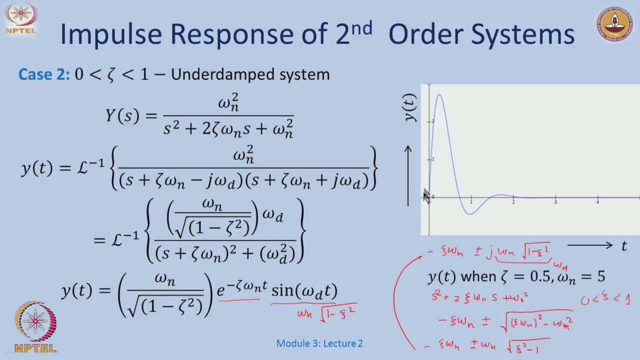 right. So we saw 3 cases now right. First is the or I actually 4 cases. The undamped case where I have the system just oscillates at the natural frequency, Then I had- well, I had oscillations, but they just die down. They die down because 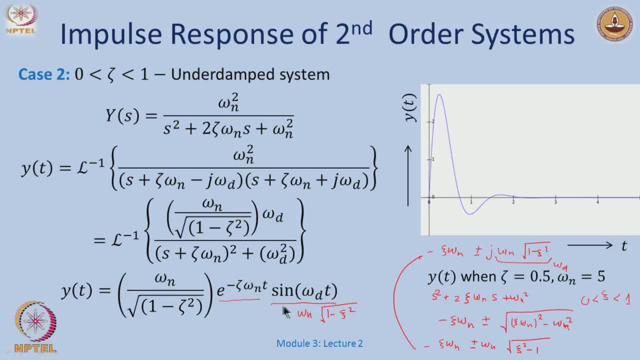 of this exponentially decaying term here. right, And this will oscillate at now a new frequency, which is which my zeta defines. Again, you can just put zeta equal to 0 and say it will again go back to the damp natural frequency. ok, And then a critically damped. 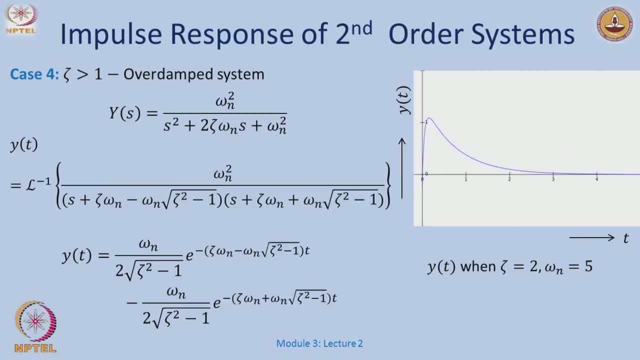 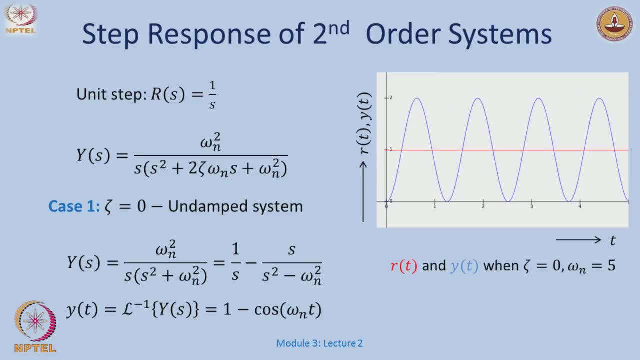 system and what we call as an over damped system. ok, Now, this was all about the impulse response. Now, how will these guys behave when there is a step response? ok, So say, The step is when my r of s is 1 over s and then y of s would be something like this: right? 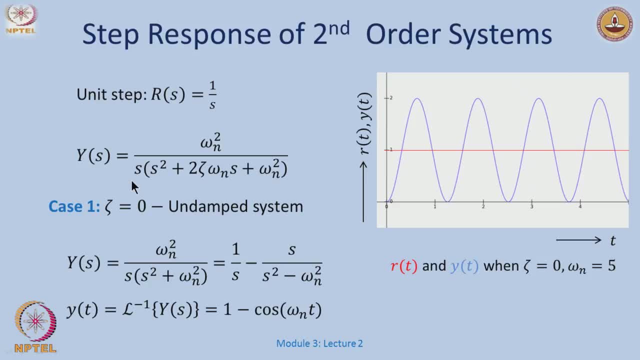 So I just have a s over here and blah, blah, blah. ok, Case of zeta equal to 0. Undamped system. well, nothing should change in principle as what was observed from the case when I had just an impulse response. So, y of s, I just do all the math and I see. well, y of t. 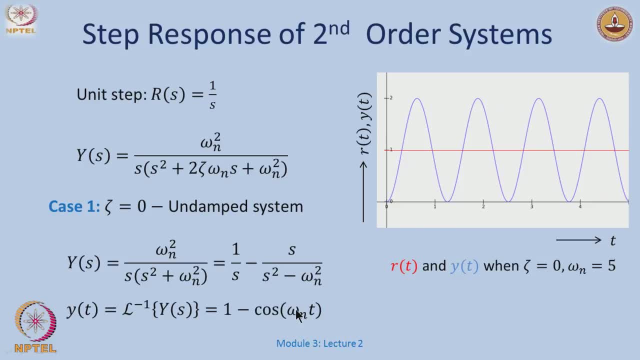 is 1 minus cos omega n t. ok, So this, Well, it is just 1 minus cos omega n t, and it will just be like this, right. And you can ask me, sir, what is a transient and steady states? Well, this guy will never reach a. 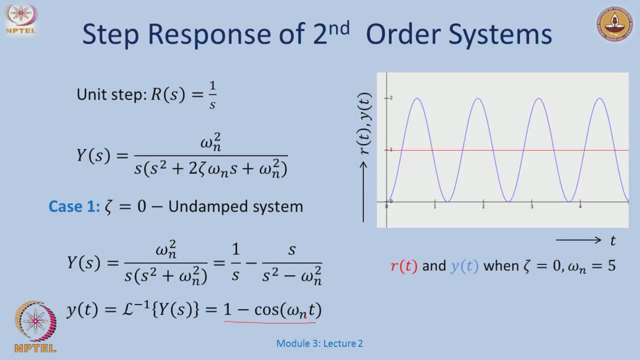 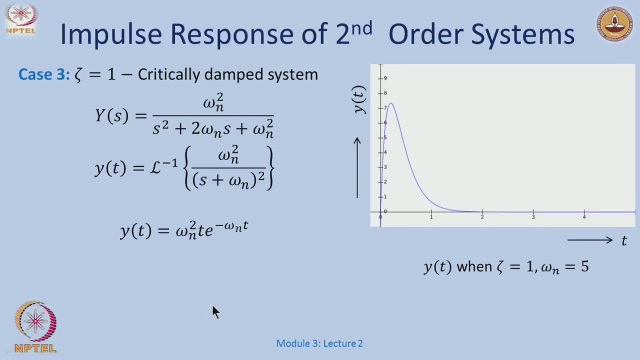 steady state correct, whereas these guys here- I just for these guys- will have, you know, this kind of transient terms which go to 0. Even the previous guy would have a transient term which goes to 0 and you see that the steady state is again. you know it is again coming. 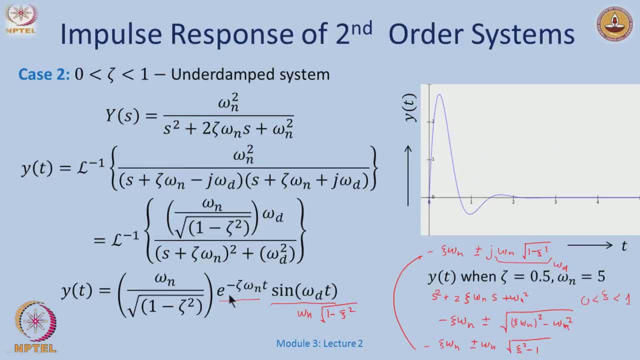 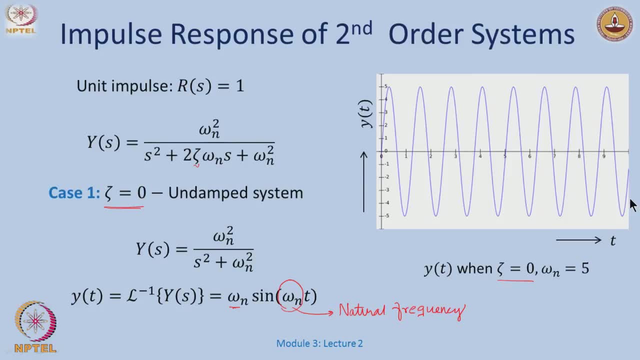 back to 0, correct. Here also, you will have the transient term, which actually is going to 0. This entire term could be viewed as a transient term and you know, the steady state term is again 0. Here, well, there is no, nothing like that, right, there is nothing which is. 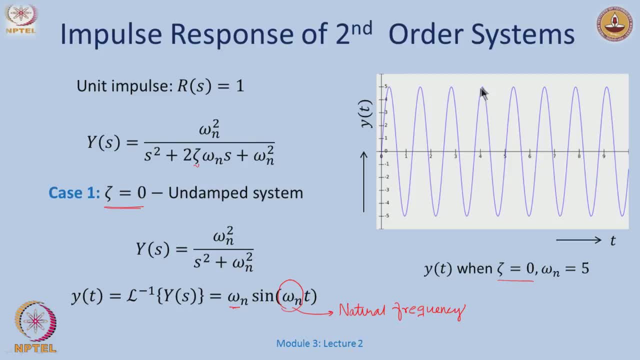 actually vanishing with time. So there is no. possibly we cannot, you know nicely- classify what is a transient and what is the steady state. It is transient behavior is actually. it is steady state behavior and it will never converts to any fixed value like a 0 or a. 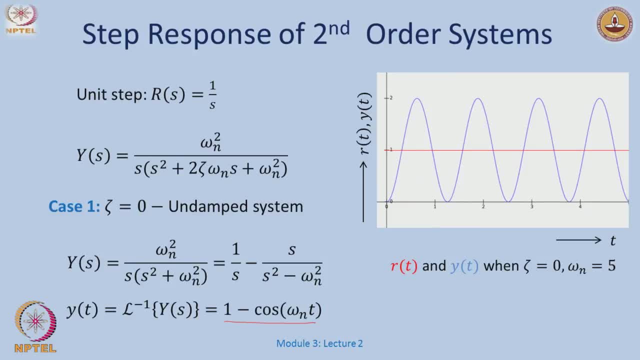 1 as in the previous case. So same thing happens when I have a unit step response. I am still doing this. one right. None of the term actually disappears as time goes to infinity. all terms are just intact. ok, This is again: zeta equal to 0,, omega n equal to 5, and the reference being a step. 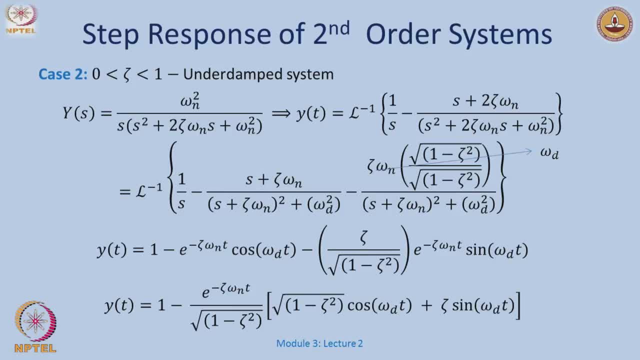 ok, Now we will do all the same cases which we did earlier. I will just skip all the math here, but we will see how my final expression looks like, right? So for zeta equal to this guy, I will, ok, start with this, and then I have this one and you: 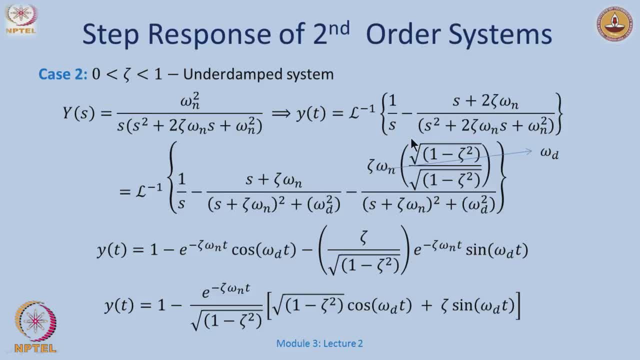 know I will of course have complex roots and all this will be taken care of here. So my response has 1 minus some exponentially decaying term. Again I have. you have some oscillating terms here which could be further simplified to look something like this: that: 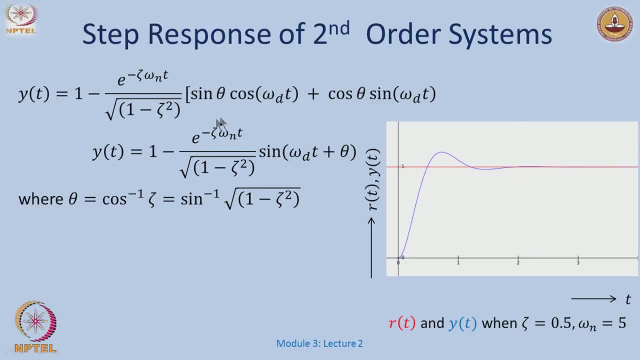 is 1 minus e power, all these exponentially decaying terms and this one, or I could call this as my transient response and this as my steady state response. right, And where theta is, we will, we will, you know. at the moment, we will just say that theta. 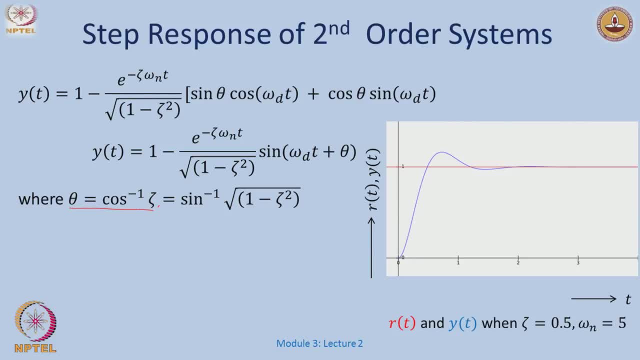 comes as cos inverse this zeta. Of course we will not really worry about why, what this means, but all the math would tell me it is just this one, right? So how does the response look? like y of t is applause. So I want to track this number. 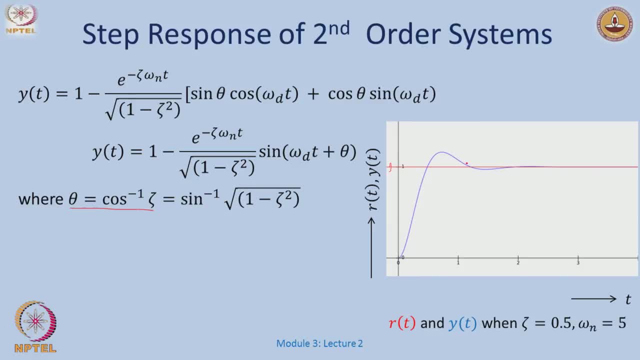 1 and I go up It into joules. So this is just enough. 1 plus omega n is equal to 1 over and overshoot, and then I go below 1 and then I eventually go to this number ok, Which I can directly say here. now I do not really need to compute what is the steady? 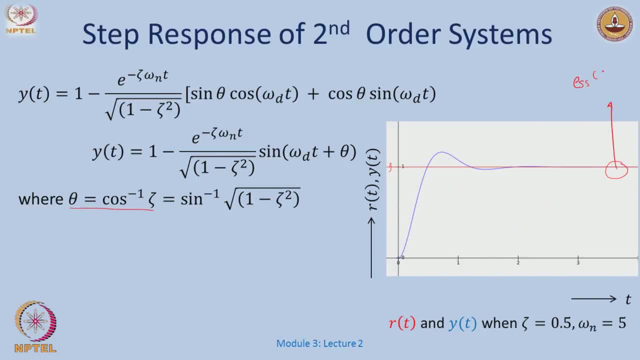 state error. just by looking at this thing, I can say that the steady state error at infinity is just 0.. We will do more analysis on this, but just as a passing observation, I am just introducing you to these terms at the moment. right, ok, And of course we can have different. 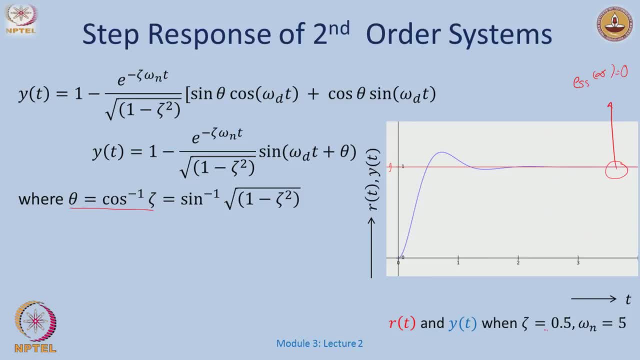 behaviors for different zeta. right as a zeta is, you know, So intuitively you can see that as zeta goes to 0, you know it is very say zeta is very close to 0, say 0.01.. Then you 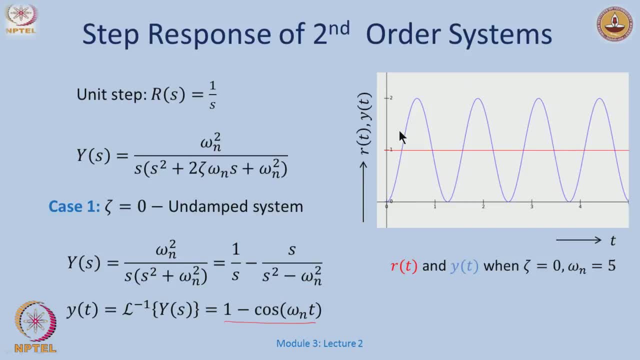 could actually expect a response which is like this: when zeta is very close to 0, you could expect and response like this, but which is very slowly decaying, right, So it might actually take a very long time to decay. So I can just draw something here and I will. 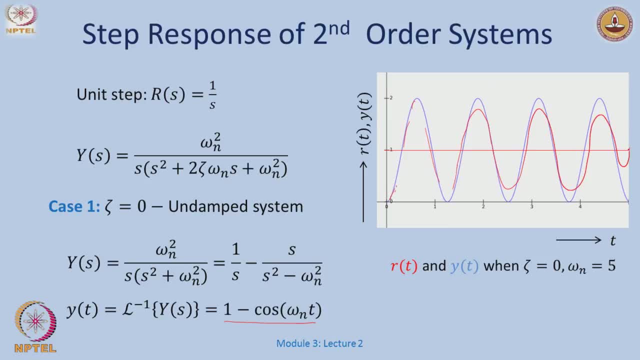 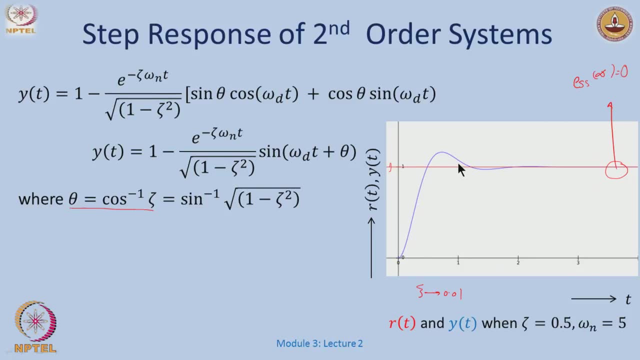 see, See these oscillations for a very long time and but they will slowly die down right. And of course, as zeta goes to very close to 1, then you will see that in the oscillations are also minimal. Again, this omega d guy just sits here right. the damped frequency of the 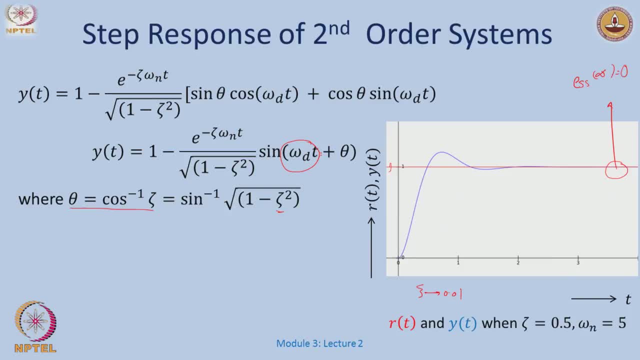 system. and this is again because of this guy, the zeta right, The justification to why we introduce this term specifically and called it the damped frequency of the system, because this is the frequency of the signal when there is and in the presence of damping. ok, 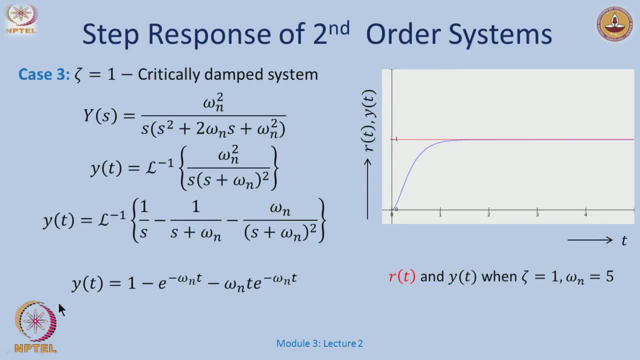 So next, what happens when I am- I am- critically damped. ok, I will just keep all this, all this math, and just see that. well, the sinusoidal terms disappear and I have just this one: y t is 1 minus e power. blah, blah, blah, blah. right, And I can just compute this response. 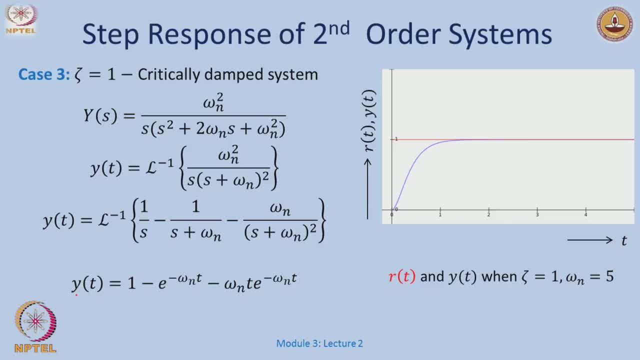 either with the final value theorem here or just put the t equal to infinity and I can just compute the error right. The error is again 0.. So this is like it goes from 0 to y in the shortest possible time and just stays there, right ok? 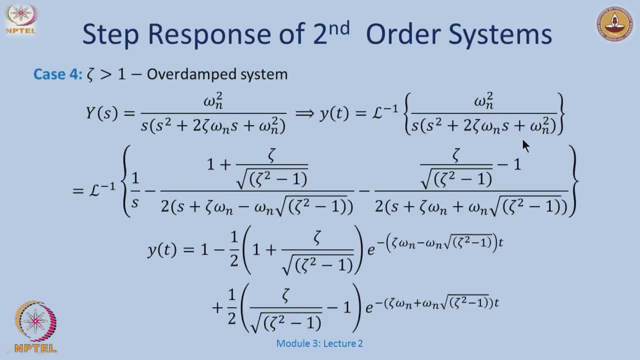 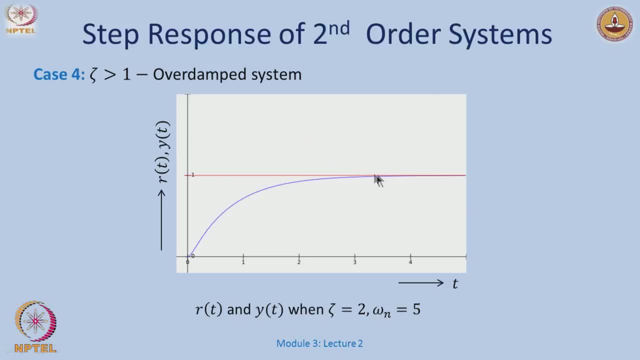 The next one is the case of an over damped system. again, we will have two exponentially decaying terms which will just be like this, right. So it will go a little slower than the previous one and you could just plot, you know things, where: if zeta goes to 3, then possibly 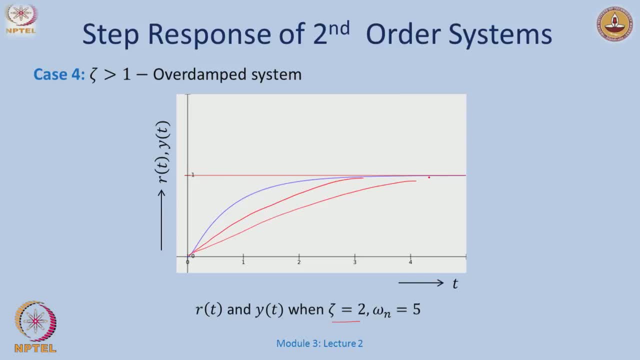 you will have a much lower response. zeta equal to 4 and much lower response. and the limiting case. we will say, well, there is a very large zeta, then you just refuse to move right. So these are also in literature. we have referred to as very sluggish systems which are like 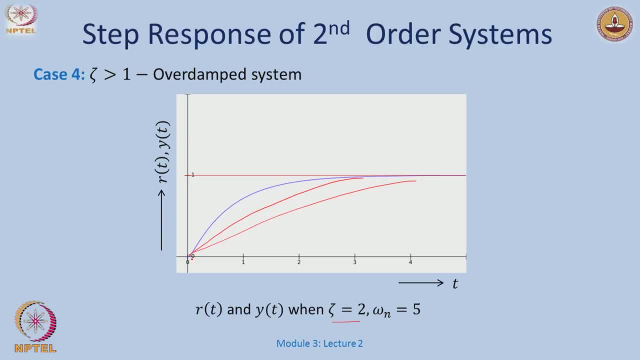 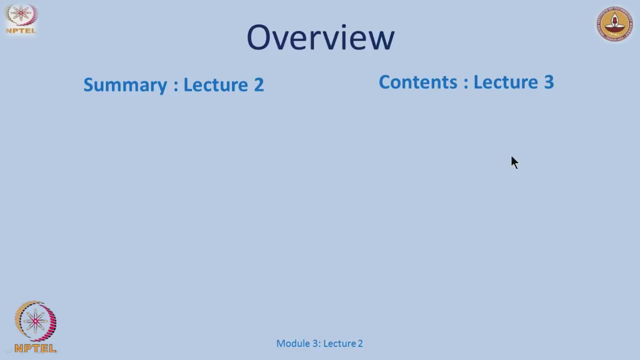 very slow to respond, right, ok, So also in this case, you can- just- you know, naturally- see that the steady state error goes to 0. ok, So what we have, we have learnt so far today is: what do we do with the models which we obtain from our previous classes? So once, 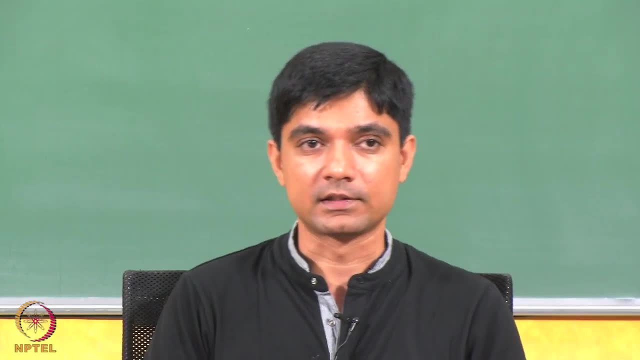 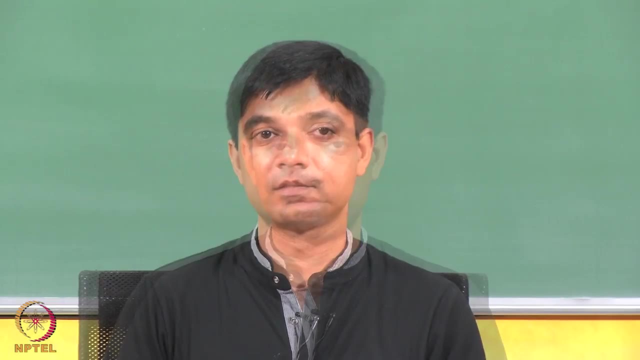 I have the models. I need to subject them to some real time conditions which I possibly would not be able to emulate in the. you know, when I am just have a system at hand, So I will just give it a certain test signals which will be closer to what I can see in. 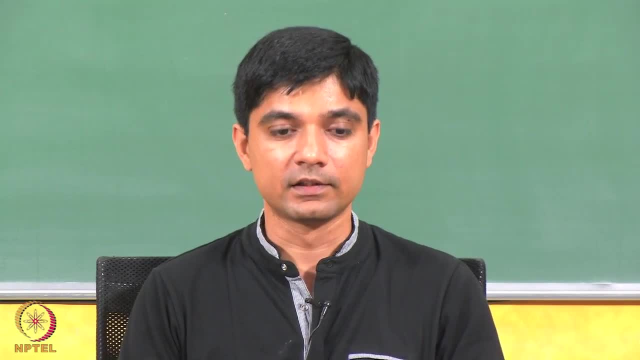 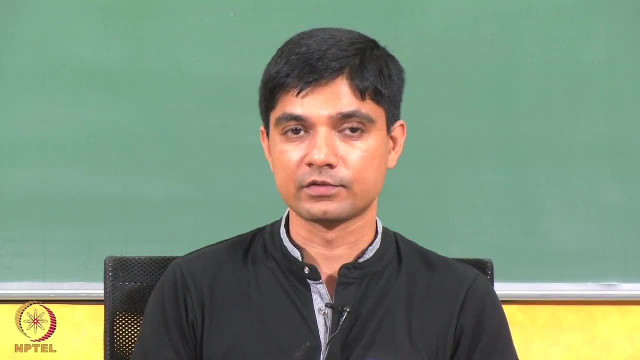 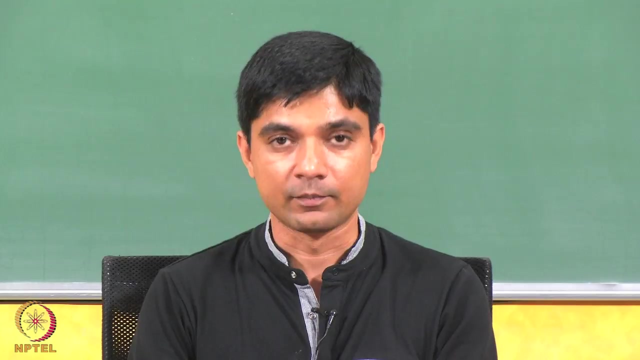 reality and therefore I have a series of signals. in my case, I have the impulse, the step, the ramp and a parabolic kind of signal and we just saw, very you know, saw what, how we could define what we call as the settling time, what are the transients, what are the? 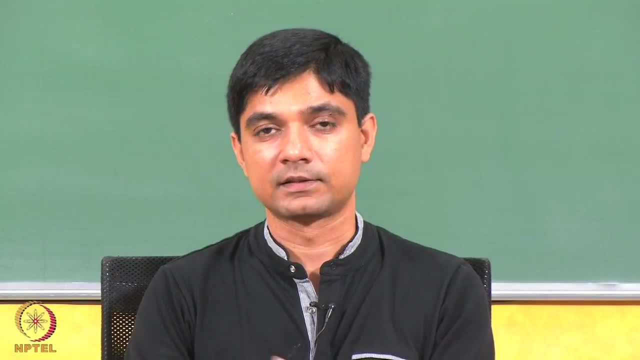 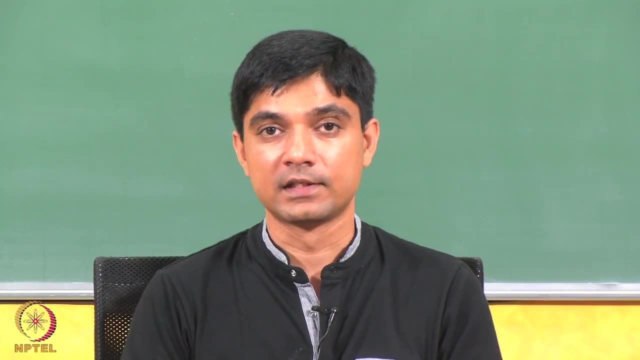 steady state And in we did it for the first order. second order case was a little more interesting because the damping actually played a role in the dynamics of the system: if I have oscillations, if I have sustained oscillations, if I have decaying oscillations or if I have no oscillations. 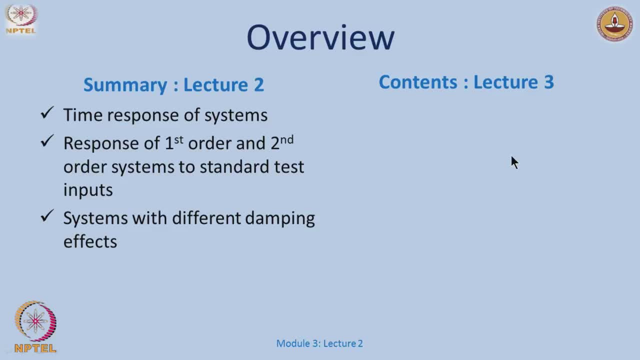 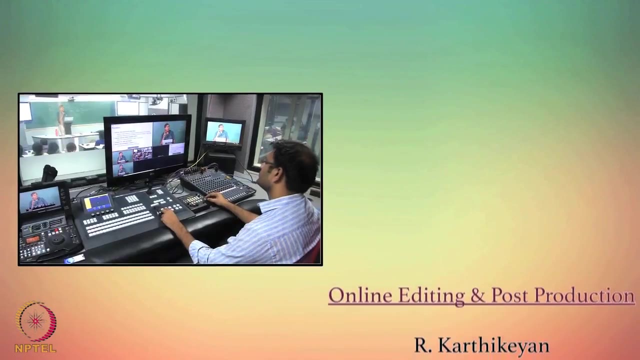 at all. right, ok, So that was the summary of what we did today and we will do a little more analysis, or we will elaborate more on this in the next lecture, when we do more analysis on this time domain specifications. Thank you.